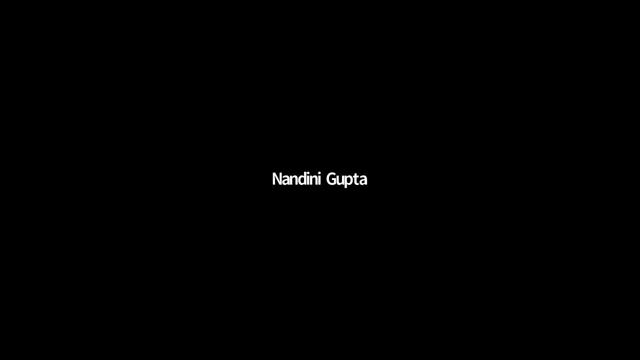 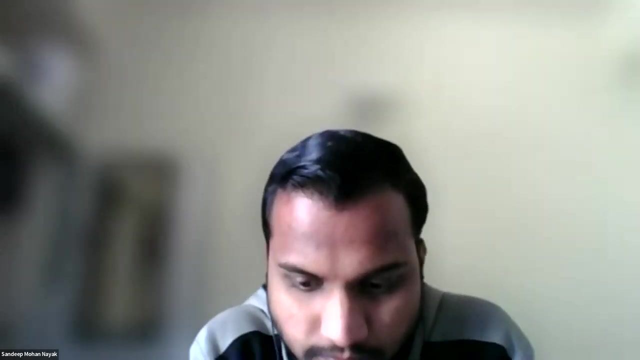 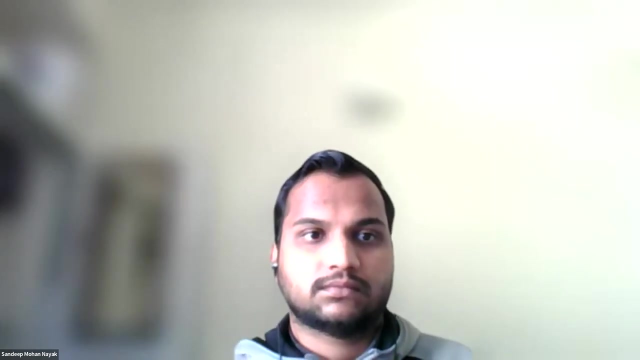 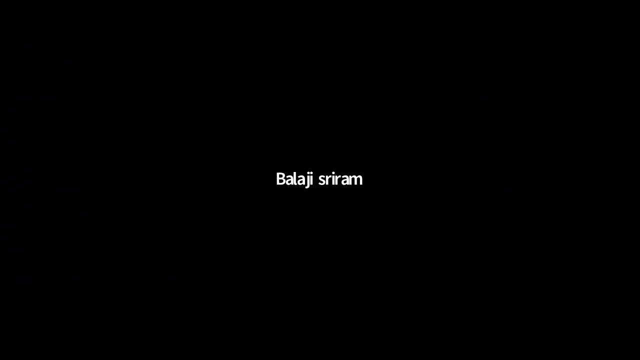 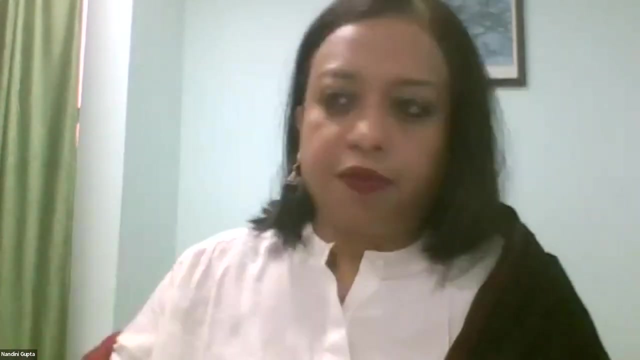 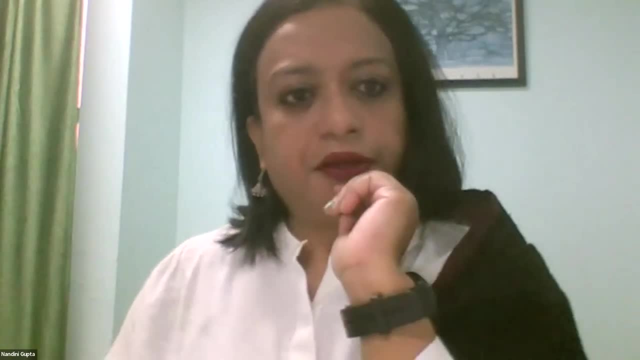 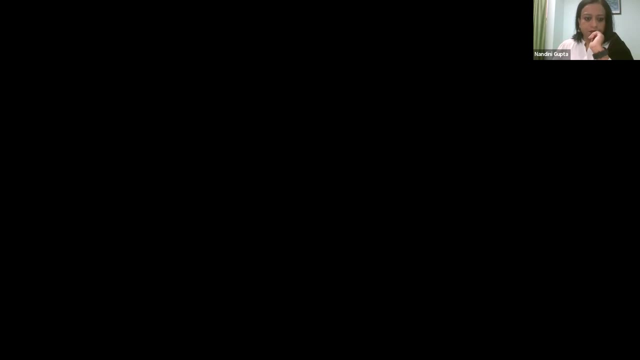 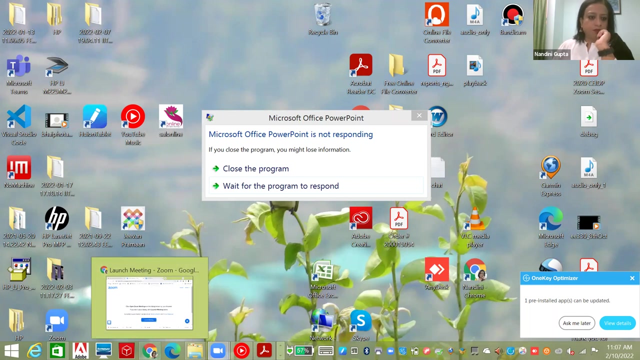 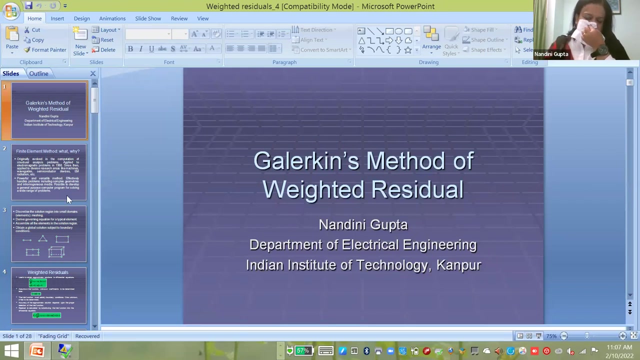 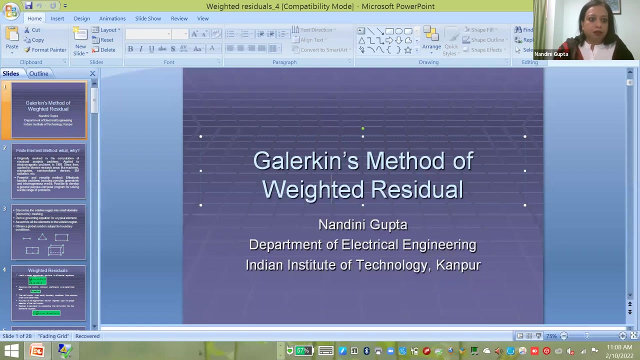 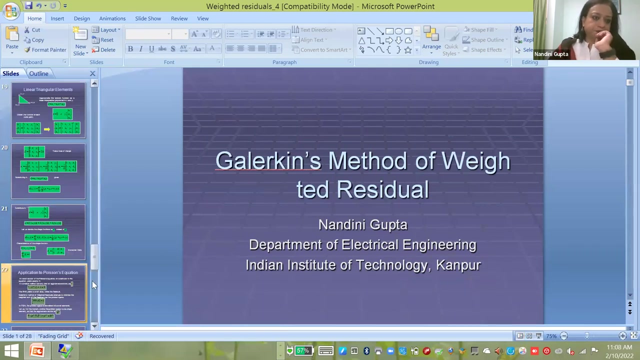 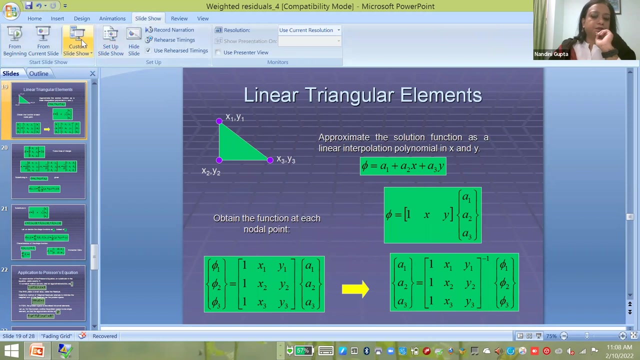 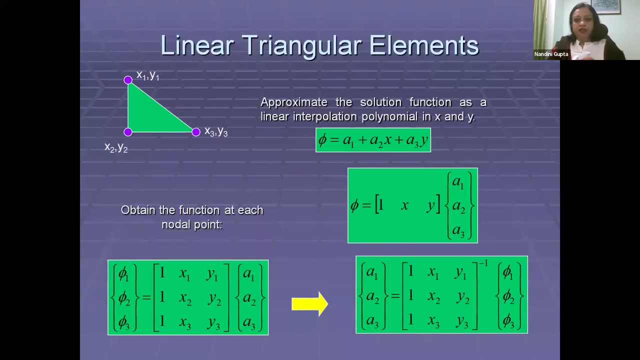 From some reason, my computer is extremely slow today. Today, I'mhard to switch the device back and forth. I'm worried about how it recognizes me. You do. Are you holding me there? Yes, Thank you, Thank you, Thank you. 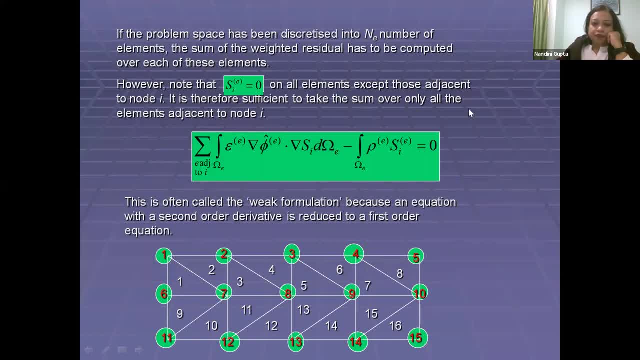 and it has been discretized into. imagine that it has been discrete, can you see it? it has been discretized into any number of elements. so let's say these are the any number of elements, which means that you will have to take the weighted sum of the weighted residual has to be taken over the any elements. so when I 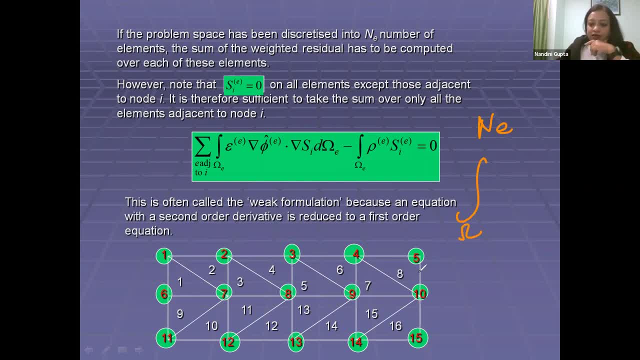 say summation, this summation has to be over the entire domain and therefore this entire domain has to cover all any elements. but we know that any shape function SI, any shape function SI is equal to zero if on any element e, if i, is not not connected to E. So, for example, if you're considering- sorry, if you're considering- 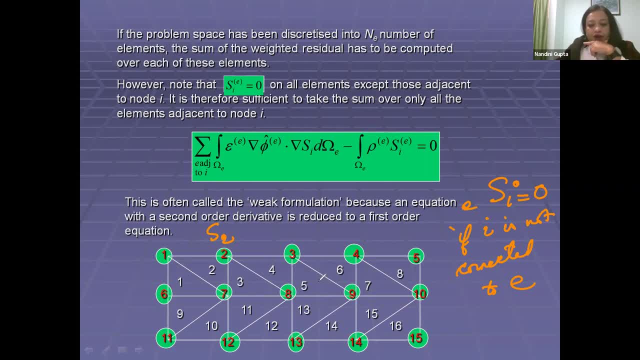 S2,. S2 will be 0 over element 5, because element 5 is not connected to node number 2.. Similarly, S1 will be 0 over 9,, 3, etc. which means that when I say that I need to take the sum, 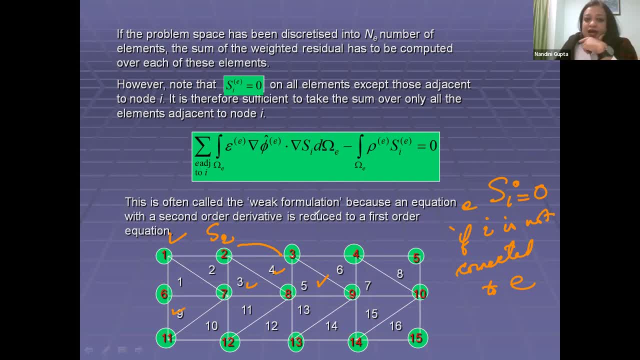 over all the elements. we actually need to take the sum over only those elements to which the particular node is connected. So therefore, on all other nodes, SI equal to 0. So if you evaluate SI and integrate or multiply or do whatever you like, you will get only. 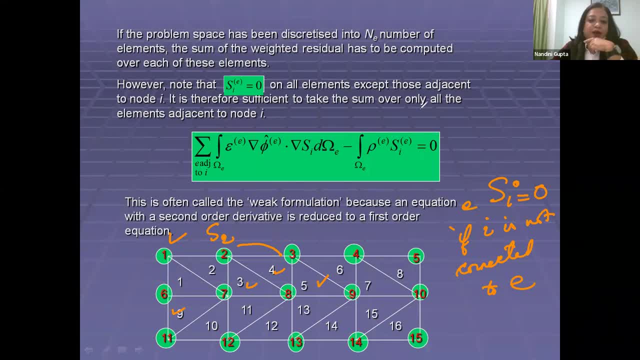 a- 0 component. It is therefore sufficient to take the sum over only all the elements which are adjacent to node I. So therefore, this integration needs to be summed by the sum over all the elements. So therefore, this integration needs to be summed. 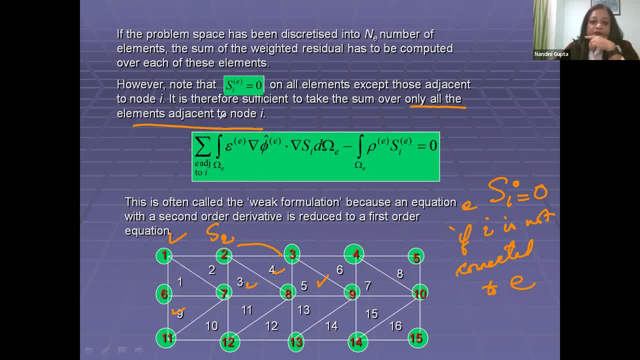 over. So this integration- by this integration I mean all this entire integration- has to be summed over all elements which are adjacent to I, And that summation has to go to 0.. Now, if you remember, in this case we have already converted del squared phi to grad phi. So 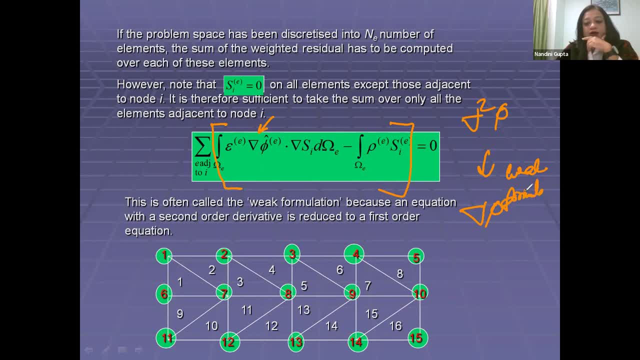 this is the weak formulation. We are going to work with del phi And we are not going to work with del squared, del squared phi. So we have reduced the highest order by one order already. So this is the weak formulation. This is what we wanted to. 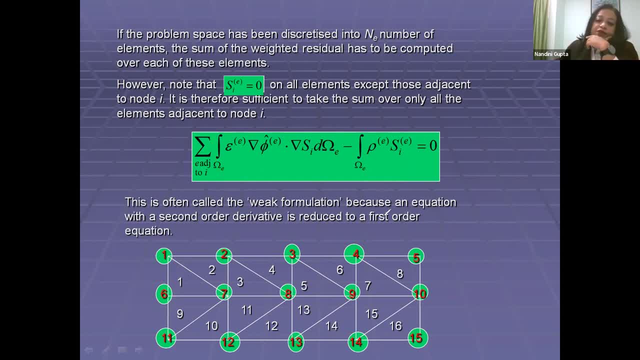 do This is also the sum of weighted method, of weighted averages, weighted residual. Now, this is an arbitrary space domain And I have taken a regular mesh of linear triangular elements. I've done this manually, just for illustration. So, as you see, these are the elements 1, 2, 3, 4, 5, 6,, 7, 8.. And these are your nodes. 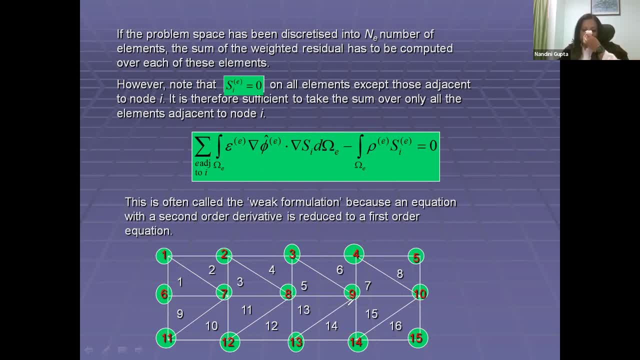 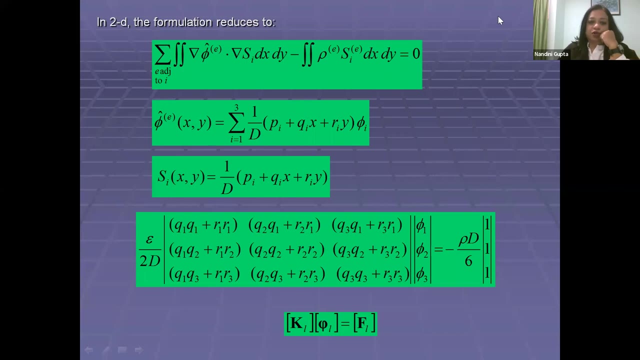 1,, 2,, 3,, 4,, 5,, 6, up to 15.. So we have 16 elements. We have 15 nodes. This is pretty simple. Let's see how we work with this Now. I want you to do this on your own, because 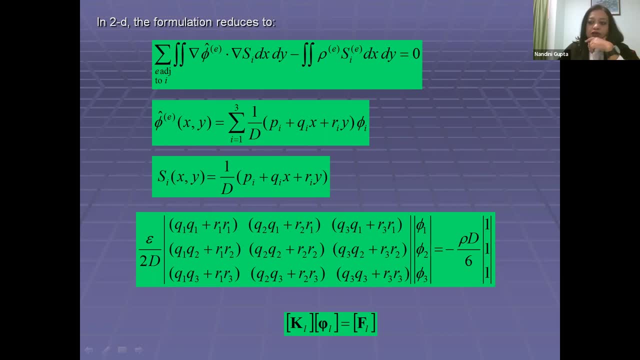 by hands, because unless you do that, you're not really going to understand what's going on. So I am going to evaluate again. This is over the entire thing. So I am going to take summation of biology. Can you do something In this PPT of weighted residuals? 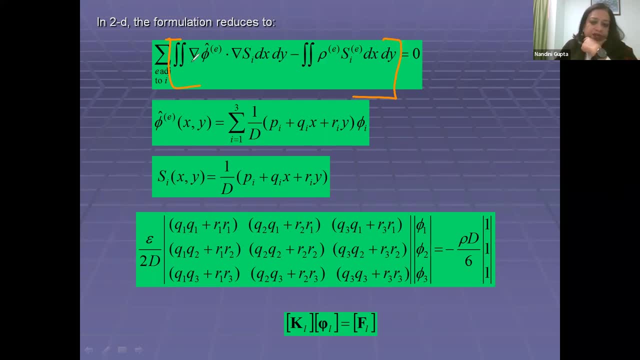 there are quite a number of errors or typos that I have been noticing while studying, while teaching. Can you note them and correct them so that you can work with the corrected version? Yes, ma'am, I'll do it, ma'am. 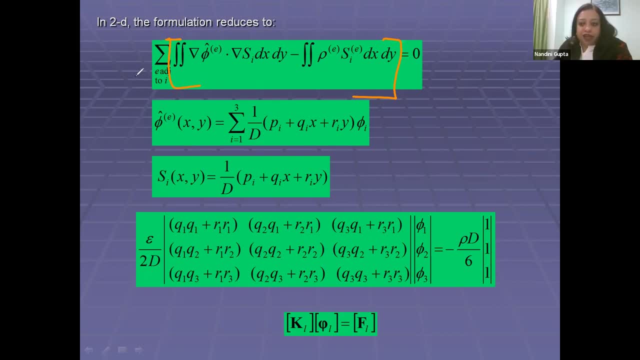 Okay, So summation, we need to perform this entire integration and then we have to sum it over, all of these adjacent to I. So let's consider a particular element E Now. in that particular element, I have summation 1, D, P, I, Q, I, et cetera, And SI is given by: 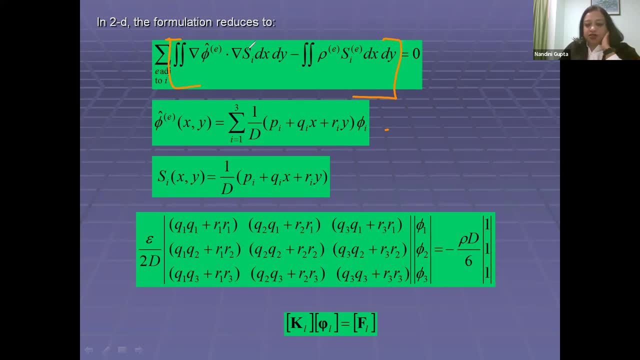 this Now, if you evaluate this integration, I want you to do it. I haven't done it here, I haven't shown the working here. Of course I have done it: Evaluate grad SI, Evaluate grad phi, And then SI. rho is of course constant, in which case this is: 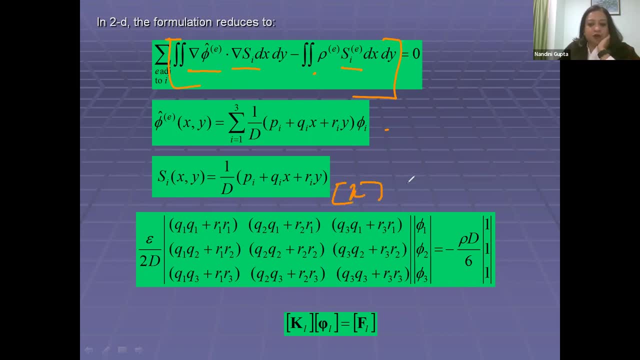 what you get as the stiffness matrix. So, as you can see, this is of the form K, phi equal to F. For the moment, you have to take my word for it, but I really want you to do it because otherwise you will be in trouble in exams. Now what I want you to note here: 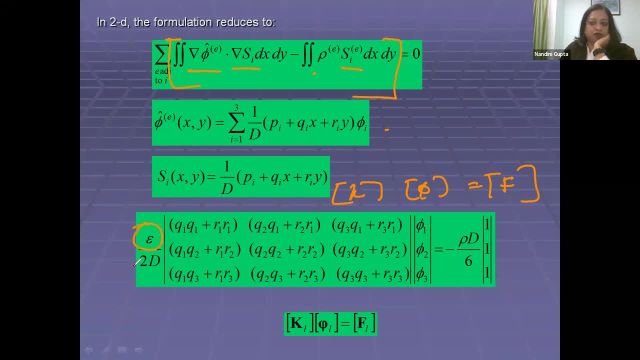 is that epsilon is a material parameter. If you remember, I have told you that for a particular element, epsilon has to be constant so it can come out of the integration, And what you have to do is evaluate R in terms of Q1 and R1.. Q1, Q2, Q3, R1, R2, R3, which means these are all. 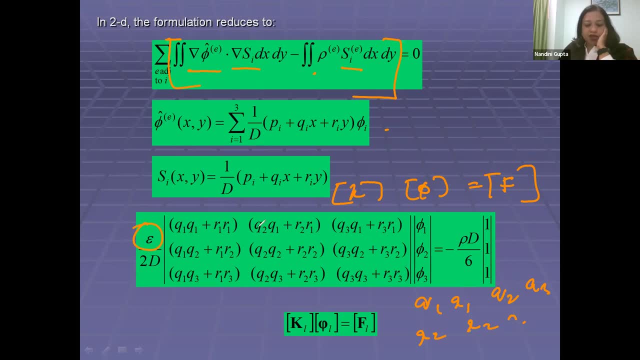 constants because they are defined at the nodes. So these are all in terms of the nodal coordinates. If you evaluate Q1, if you evaluate R1, R2, Q2,, all these R can be evaluated in terms of constants. So for this particular problem, you will get a stiffness matrix which is composed: 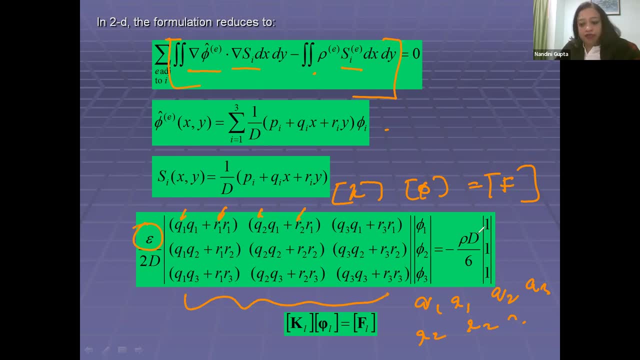 of R1,, R2, and R3.. And you can evaluate it without even using numerical method. And on this side you have phi d rho d by 6, 1, 1, 1.. So this is your local stiffness matrix. 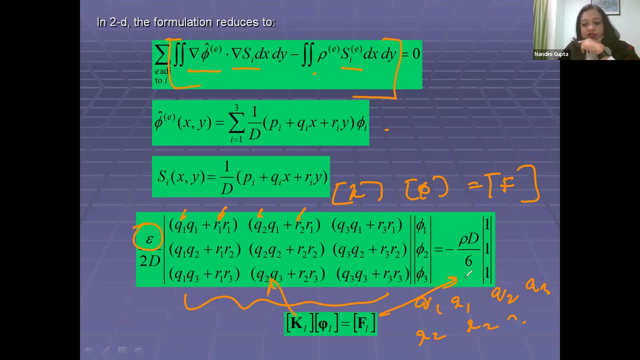 This is your local stiffness matrix. Sorry, this is a local stiffness matrix. This is your local force vector And this is your nodal vector for a particular element. Anything, any problems so far. You will need to evaluate Q1,, Q2,, etc. I have given you the expression. 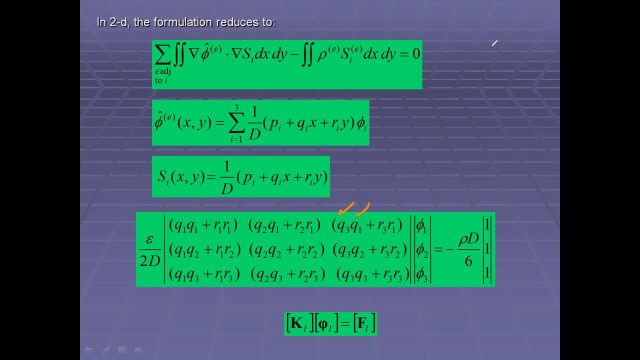 for Q1 in a previous slide. You can find it for yourself. Are you clear about this? Because I have to talk about something very important now. So your next assignment would be after you have completed the one that has been given. 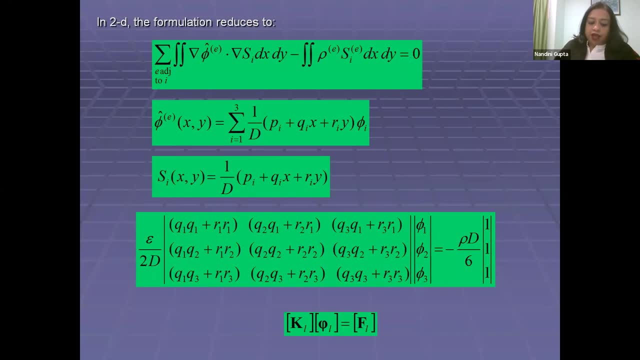 would be to write a two-dimensional program. in terms of k, phi, in terms of of PQR, you can evaluate the shape function. so, whatever program you write in one dimension, you can easily extend it to two dimensions and in that case the shape functions can be. 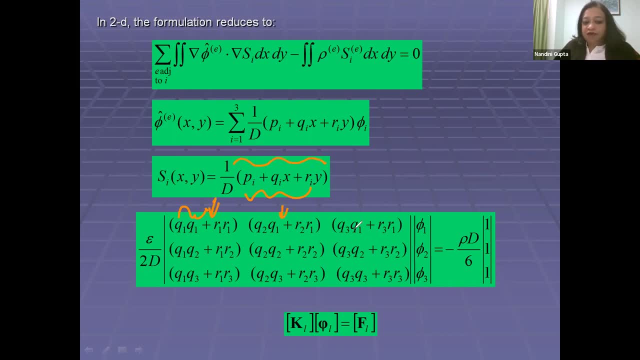 evaluated like this, and these shape functions can be here. I have not evaluated the shape functions, but I've evaluated the stiffness matrix in terms of the shape functions. you can also evaluate the shape functions and evaluate the integrals. whichever way you like, you can evaluate the stiffness matrix and, of course, you know this is the local matrix, so then you'll have to. 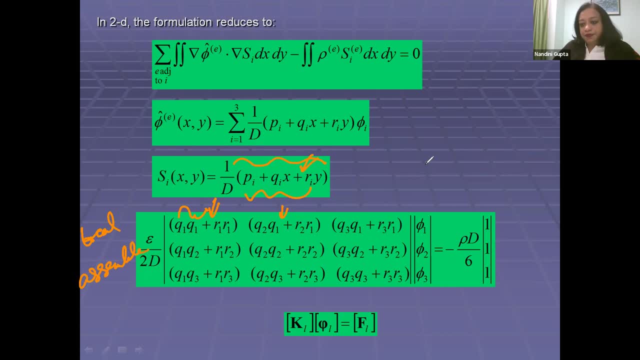 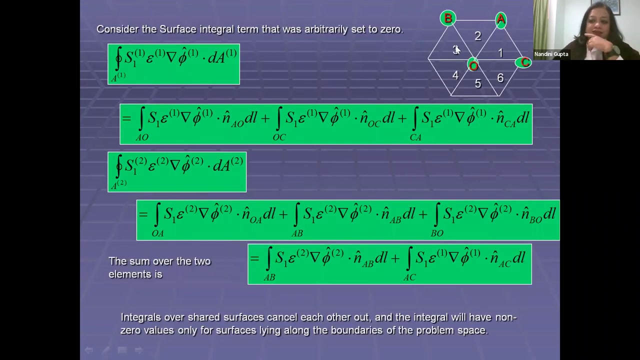 assemble it into the global matrix. so can you do this? if you had an assignment like this, are you in a position to do this at the moment? yes, okay, so next. let's go on to the next slide. now, if you remember, as Sandeep asked me, why are? 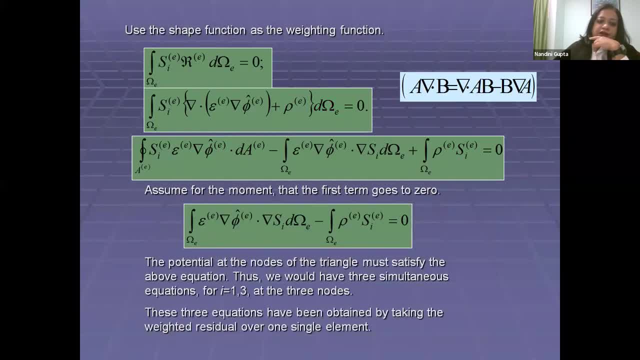 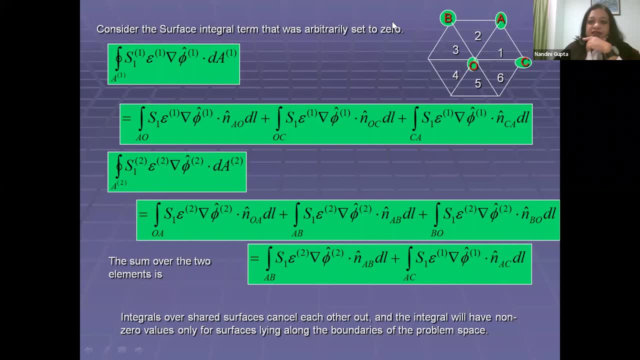 we considering the first term, to go to zero. let us see what I've done here is I've taken a special case, The special cases. I've taken a mesh. I have taken a mesh such that you have node zero or node O, which is at the center of six elements: One, two, three, four. 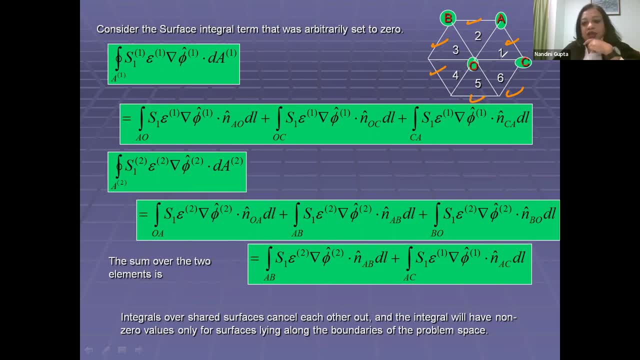 five, six And these are your other nodes- A, B, C, D. We don't need them, etc. So you have six elements. So you have a node which is common to all the six elements And these elements also. 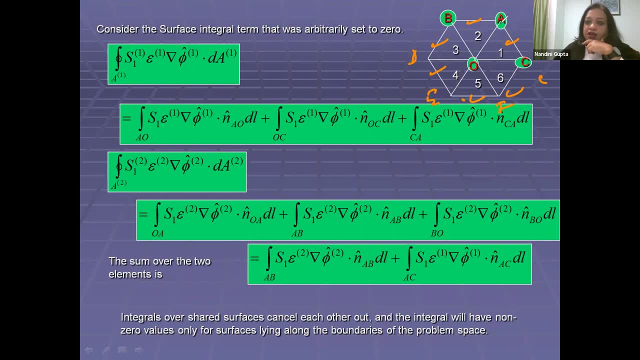 have some edges which are common to each other, Clear so far. Now let us take this first term that we have ignored for the moment. Remember, it's a surface, It's a contour integral. if you remember, We had a volume integral or a domain integral And, by applying Green's theorem, we 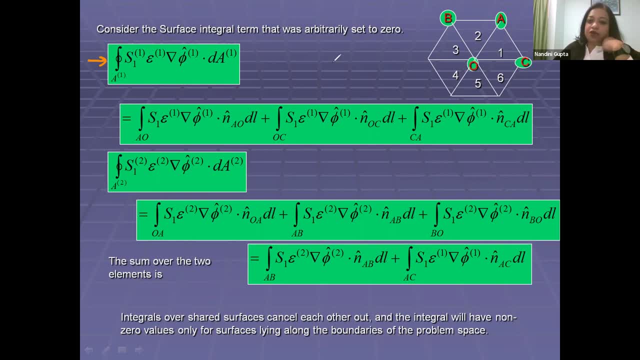 convert it into a contour integral. So it has to be evaluated. So if it's a two-dimensional situation, your volume- integral or integral over the domain- converts into an area- integral over the area And correspondingly, if you have a contour integral, the contour integral will be. 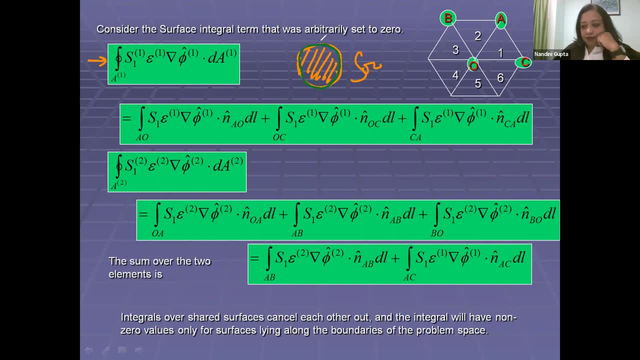 taken around the surface Right. If you have a three-dimensional volume, then your surface integral has to be taken over, just as we did in case of Gauss. It has to be taken over all the faces, But we have already reduced this. So when we are considering the volume integral, the volume in the Z direction. 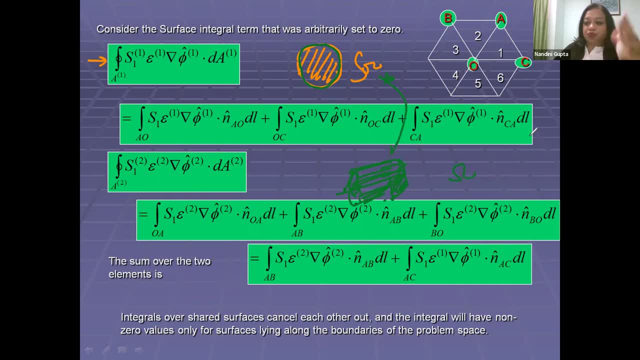 is assumed to be unity, because we are assuming that this cross-section is repeated in the Z direction infinitely. So we just have to evaluate the area integration. So we have to evaluate this. So for the contour integral, we just have to go around the domain That is your contour. 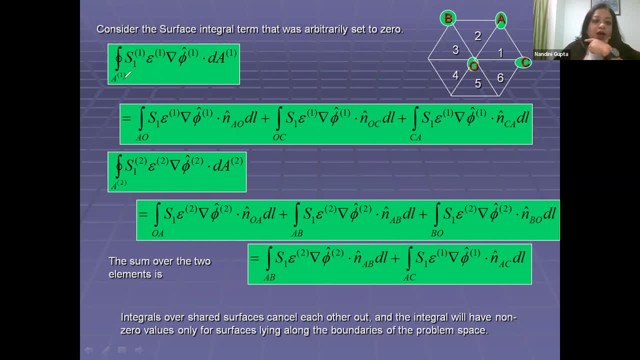 integral. So that is what we are going to do here. Now let us imagine that we are considering element number one. In element number one, the first term, the first equation will have S1.. I am only considering the first term, So the first term in 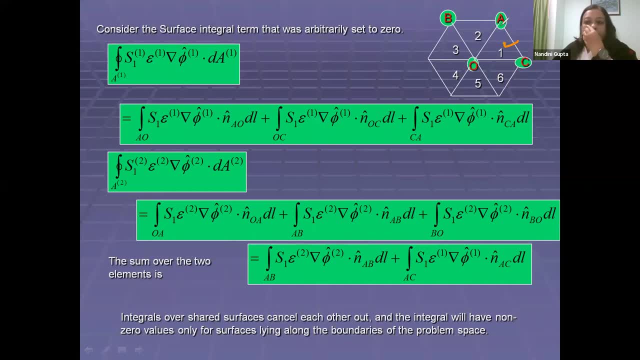 In terms of the shape function at node number one. let us call this node number one. Let me see. Let's see One, two. Okay, I'll see. I can't remember what. we have assumed which to be node number one. I'll do it as I go along. So I need to evaluate S1 over element one, epsilon over. 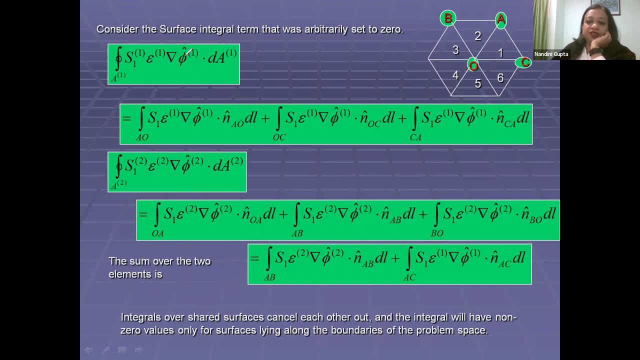 element one grad phi over element one. See, this is the tilde, so it's a trial. So I need to evaluate S1 over element one, epsilon over element one, grad phi over element one. See, this is the tilde, so it's a trial. 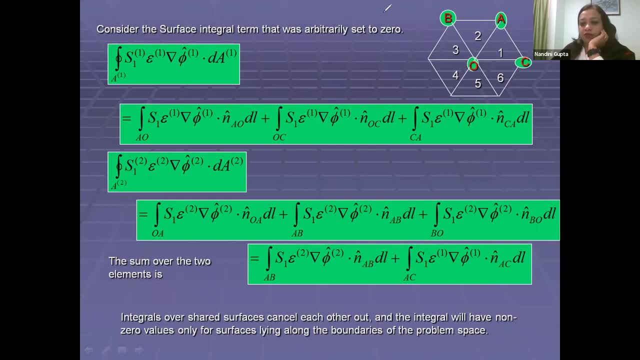 I need to evaluate this function into DA1, so area of element number one. So we are talking about this element. When I want to evaluate this and I want to take the contour integral, what should I do? So I have to take integration over this edge: OC, CASCA and AO. 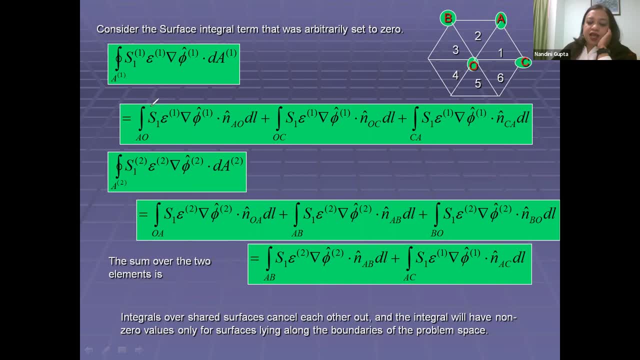 So therefore I break this down into three terms: is inside remains the same: S1, epsilon, grad phi, dot, the normal along AO and the normal along AO. So this integration converts into the integration of this integrant, over this edge only. So we consider the normal along this plane, along this face, and we integrate. 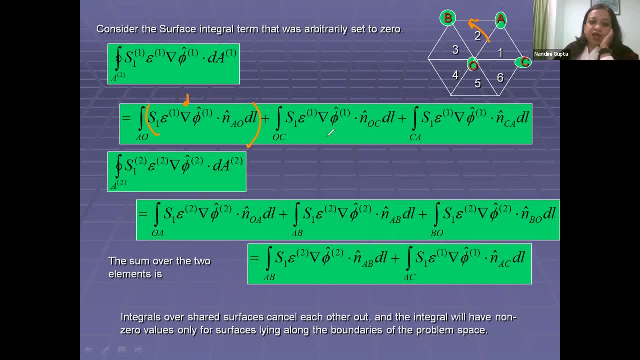 that. So we integrate it over here. So this is the first term. Second term is OC, So over here, and this is your NOC, So dot, NOCDL, And then you have this term. So when you integrate the same quantity over this edge, we take the normal outward, normal of this edge outward. 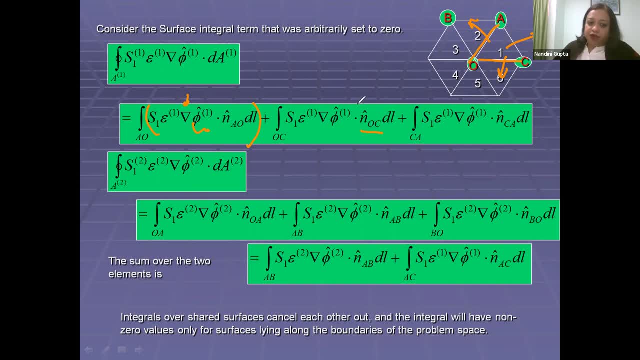 normal of this edge, outward normal of this edge, and we perform the integration. This we have done. let's say Now we would have to perform the same integration over element 2.. So let's say this is node number 1. In that case element 2 will also have- or let's say this is node number 1.. 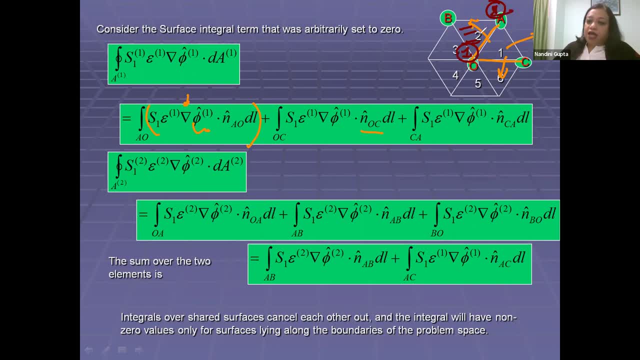 So element 2 will also have. element 2 will also have contribution from S1.. So S1 will not be 0 on element number 2.. So S1 will not be 0 on element number 2.. So S1 will also have contribution from S1.. 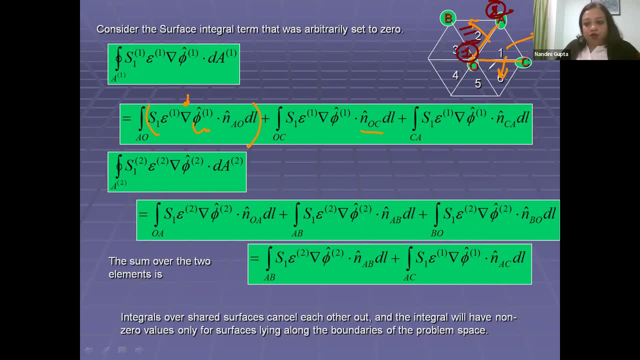 S1, terms containing S1 will also have to be evaluated over element number two. So when we do the same thing over element number two, again we have the second, first term which we have ignored. Difference with: it's the same term, except now we are taking S1, that part of S1, which is over element number two. 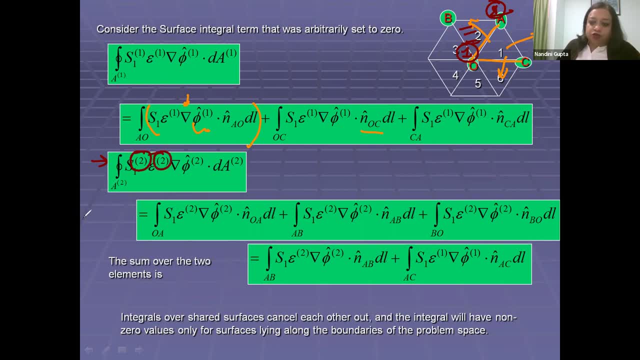 We are taking the permittivity of element number two, So the permittivity of the material parameters in element one and element two can be different Grad phi over element two. So the trial function, remember, is different over different elements. and then the area of element number two. 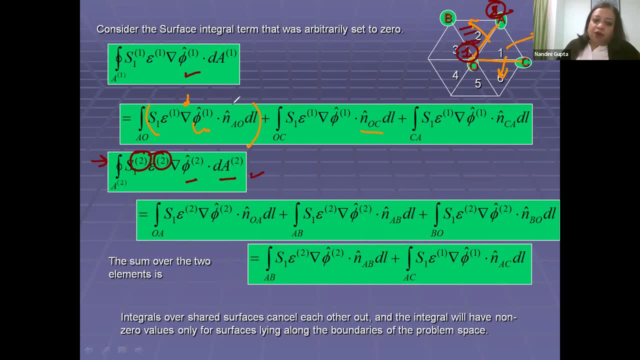 So we are performing the same integration, but now we are performing the integration over element number two. So of course, S1 will have a different value. Grad phi will also have a different value Again, since this is a contour integral. now I will have to perform integration over these three edges. 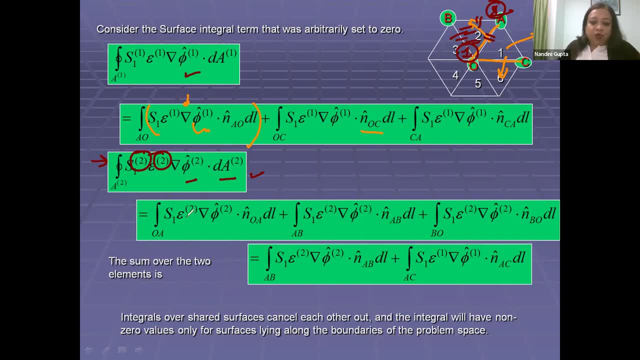 So let me break this up into these three edges: S1, epsilon, S2, grad, phi, S2, dot, NOA. What is NOA? NOA will be now the sub outward from this element: NAB, NBO. So, if I look at it, what I'm having to do is I have these three normals, over which I am integrating the terms of element number two. 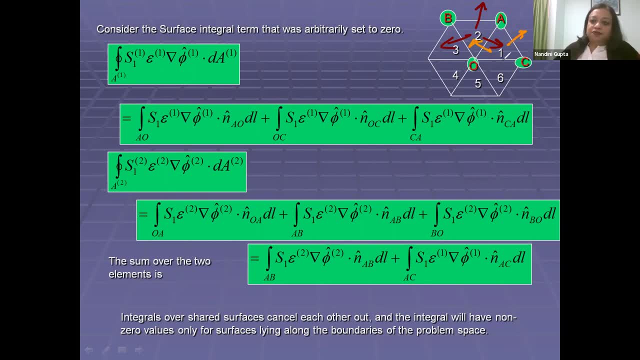 And earlier I had These normals Which I over which I had integrated the same term. Now, if you remember something, We have continuity of the solution Over elements. So when I pass from one element to the next element, the solution has to be continuous. 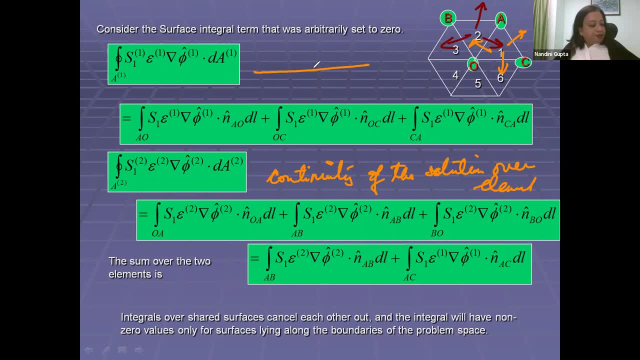 What does that mean? It means that at the edge the element has to add. the solution has to be unique. You have two solutions. You have solution one from elements number one and you have solution two from elements number two. But at the interface between elements number one and elements number two, phi one and phi two have to be equal. 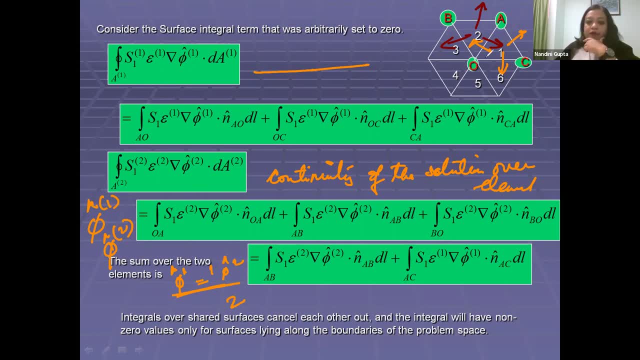 You cannot have two values. So therefore, In that case, look at these two terms, This first term and this first term: S1- S1.. Epsilon one, epsilon two. You can take epsilon one out, Grad phi one, grad phi two. 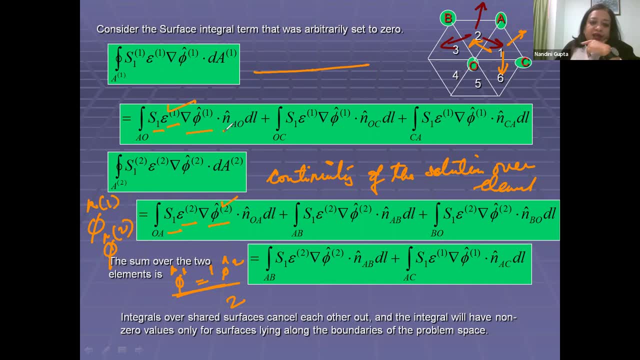 We don't know anything about it. And then you have The same thing being integrated over NAO And Integrated over NOA. So At the edge, the grad phi has to be the same. and forget about epsilon, because epsilon is a constant, therefore it can be taken out. 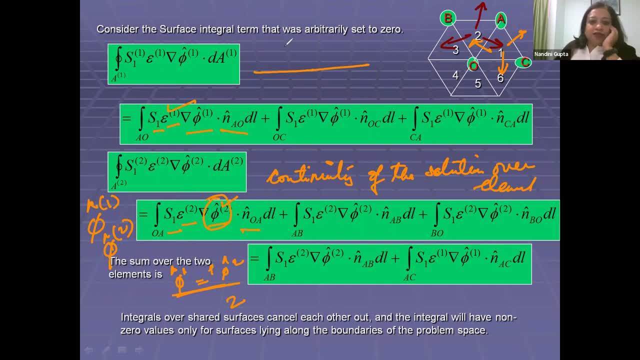 So what are you left with? You are left with S1 and grad phi one, S1 and grad phi, and both of these must be equal at the edge. And what are you doing? S1, grad phi- five Is The same quantity at the edge. 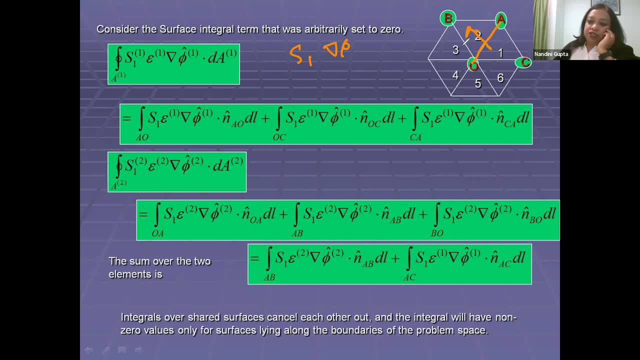 Once you're integrating it by multiplying with this normal. The second time you are integrating it by multiplying with this normal, Which means they must be equal and opposite. Therefore this term, when I add these two terms together. So if I take the left hand side of the right hand side, 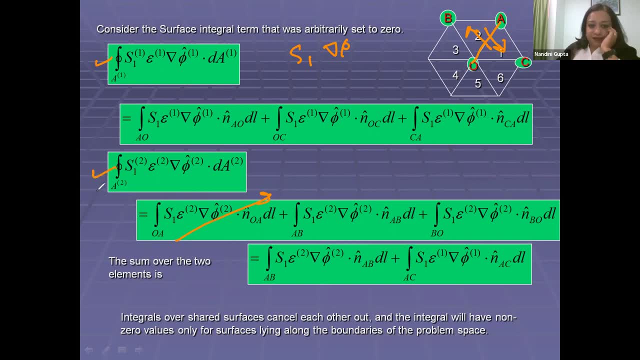 I took out other. So this plus this, Let's add LHS1 plus LHS2.. So I will have these three terms and I will have these three terms. Out of these three terms, this term will go to zero, because this will cancel this out. Similarly, if you look at CA, you are going to evaluate CA and 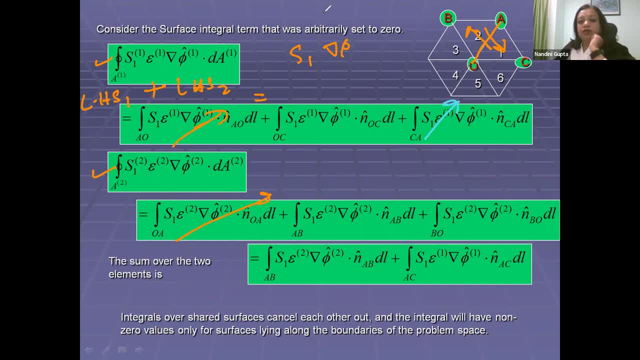 you're also going to. where is CA? No, no, sorry, not CA- OC, OC. where is OC? Yeah, Okay, let's consider these two terms only. So, in these two terms, when you add LHS1 and LHS2,. 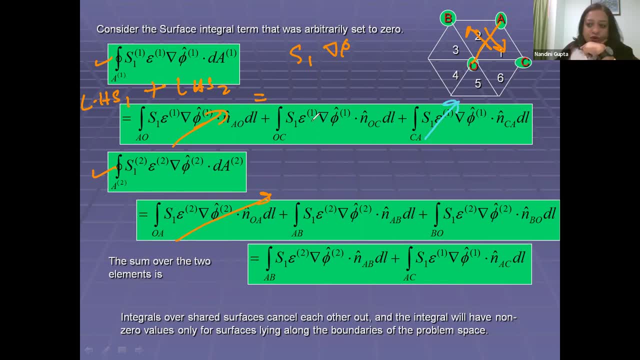 the common edge cancels out. So you are left with an integration that has to be performed over this edge. Right, You do not have to perform this integration. You only have to perform integration over these edges because of the first term. So the first term has to be evaluated over the. 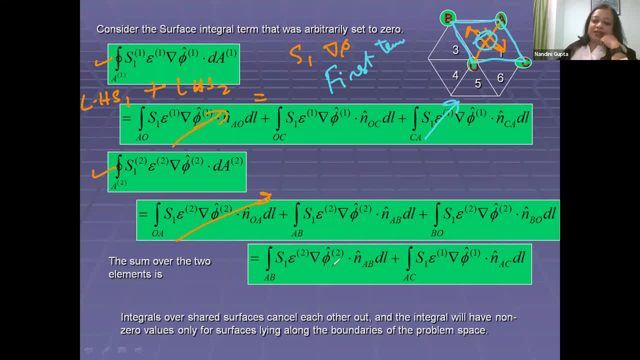 outer edges of these two elements. Now let us take this other case. Let's take the case where we consider element number six. When you have element number six, this edge will cancel out between one and six. Similarly, if you take five, 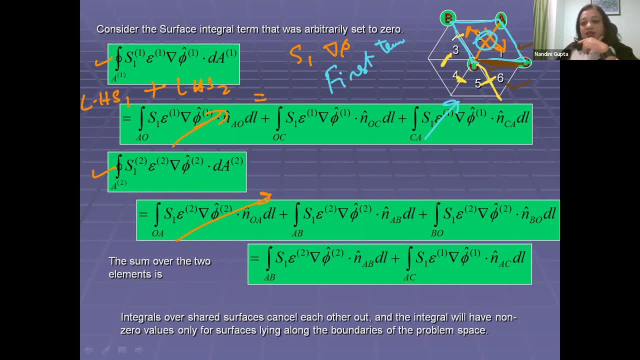 this edge will cancel out. this edge will cancel out. this edge will cancel out. So, as you keep taking two adjacent sides, the first term evaluation of the first term over the internal edges did not be performed, because this will cancel out this. this will cancel out this. 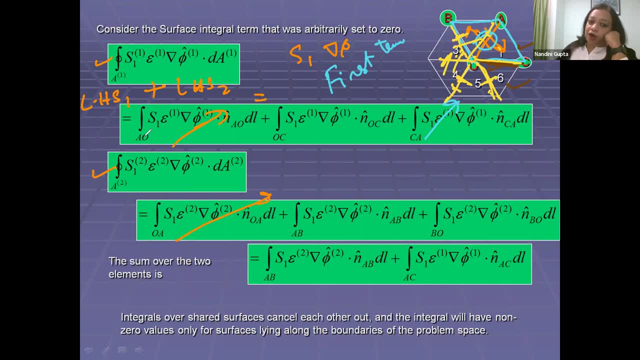 this will cancel out this, and so on and so forth. So you can just forget about the terms which need the evaluation of this integral over any of the internal boundaries. Is that clear to everybody? So what will you be left with? You will be left with the integration of the first term. 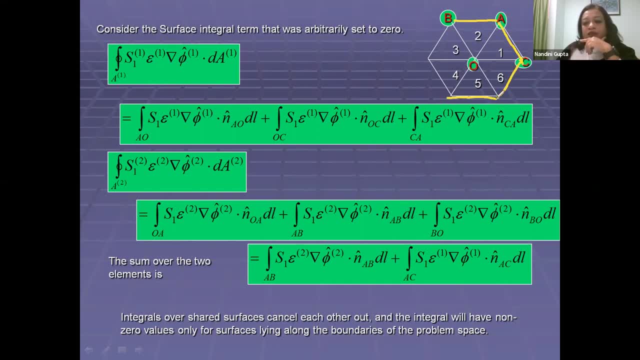 which has to be evaluated over only these external boundaries. Is this clear to everybody? And we are considering the permittivity to be equal? no, No, it's not necessary. Epsilon comes out. Epsilon is constant. Okay, for the moment. yes, let us consider. Okay, I'll come to that point later. For the moment, 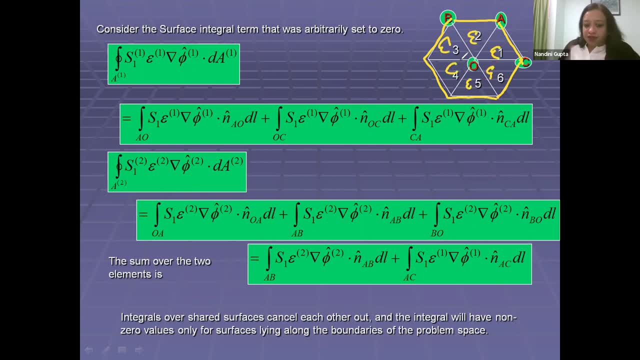 let us consider epsilon to be constant everywhere. Yes, let's consider that For the moment, I'll tell you what happens when epsilon is not constant. I'll come to that later. For the moment, yes, epsilon is constant. Only then, at the moment, you'll be able to cancel out total. 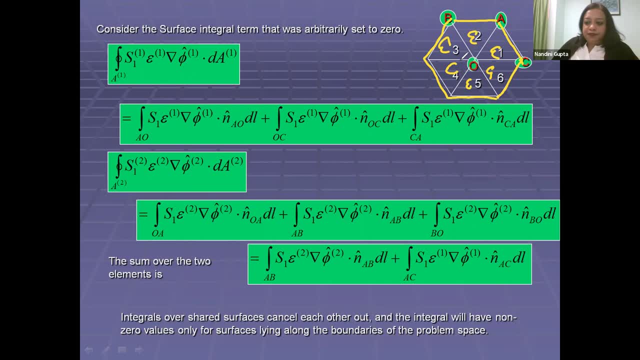 And then you'll be able to do that. But when epsilon is not constant, you'll be able to calculate the. What about the others? Deja Girish. Yes, ma'am, What did you understand? Yes, ma'am, it's not good enough. 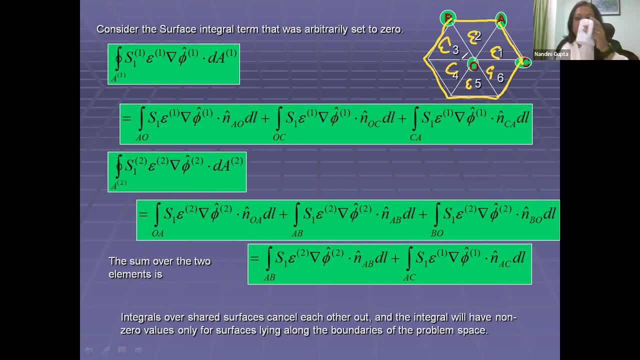 What is it that you understood from what I just explained? Tell me in one word, in one sentence: Shaded surfaces will get cancelled out, ma'am, and will remain with only the outer surfaces. Okay, Now, Hello, Yeah, Who is that? 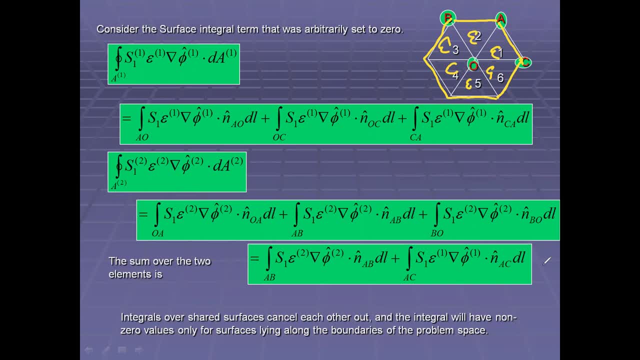 Ma'am in the epsilon, Ma'am Girish, Uh-huh. yeah, Ma'am in the epsilon. That's why I say please switch on one minute. That is why I say switch on the camera, at least when you speak. 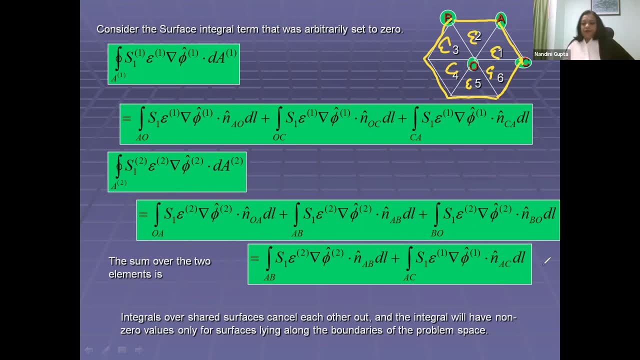 because then I can see you immediately. Okay, tell me, Ma'am, in the epsilon, in the element one and element two epsilon are different. Yeah, for the moment, I have asked you to consider How it can be cancelled. 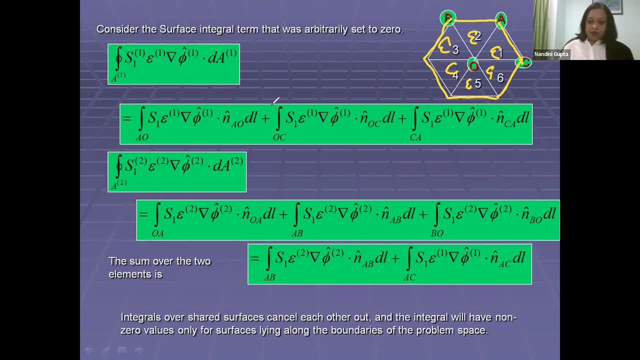 For the moment. I have asked you to consider, I have asked you to consider the same element, the same permittivity. Okay, okay, ma'am. Any other questions? Okay, so, So, this is what I wanted to say. 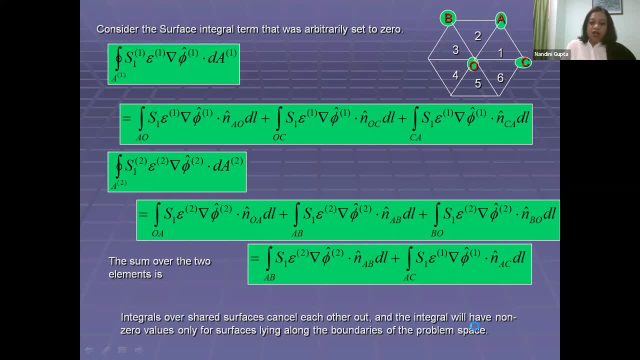 integrals over shared surfaces cancelled each other out and the integral will only have non-zero values. Four surfaces lying along the boundaries of the problem space. See, I have taken six elements. You can imagine there are a large number of elements Even if you have a very large number of elements. 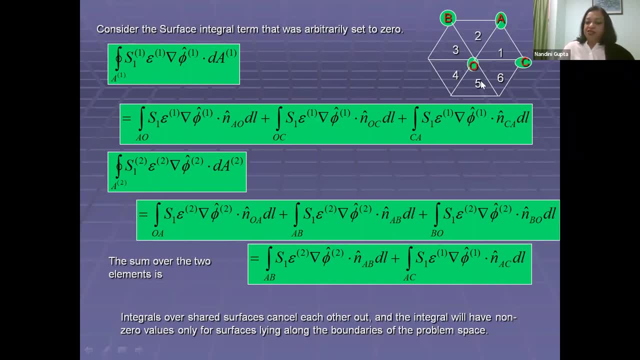 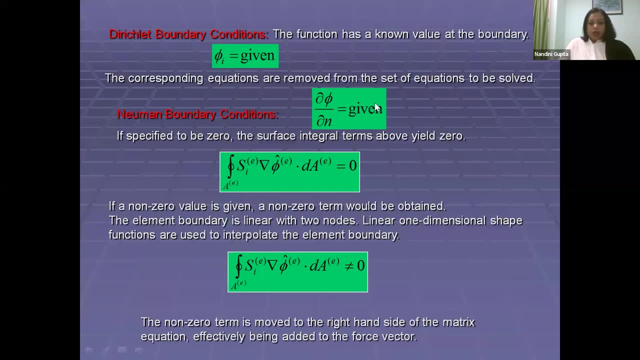 large number of elements. whenever there is a shared surface, the integral will cancel out and you will be only left with the outer boundaries. Now, when you have, let me go off at a tangent and explain something that you already know. when you have to evaluate a solve, what is happening? 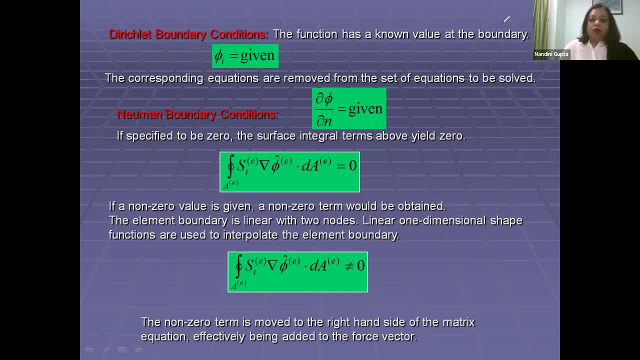 when you have to solve a partial differential equation. it is subject to certain boundary conditions, and these boundary conditions can be of two different types. One is that you must have learned this somewhere. one is the Dirichlet boundary condition and the other is the Neumann. 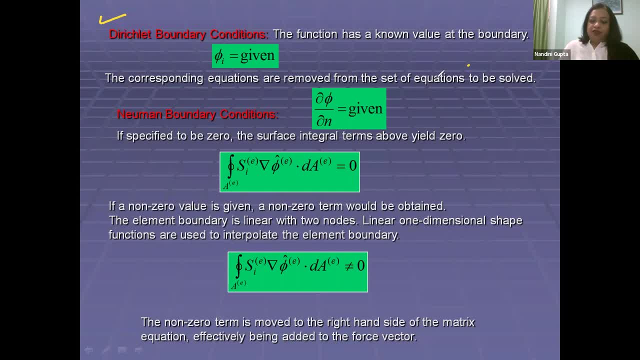 boundary condition. In the Dirichlet boundary condition the function has a known value at the boundary. So the example problems that we worked out in one dimension, we have to solve them in the Dirichlet boundary condition, Where I said that phi one is equal to, not phi one we were working with u one is equal to. 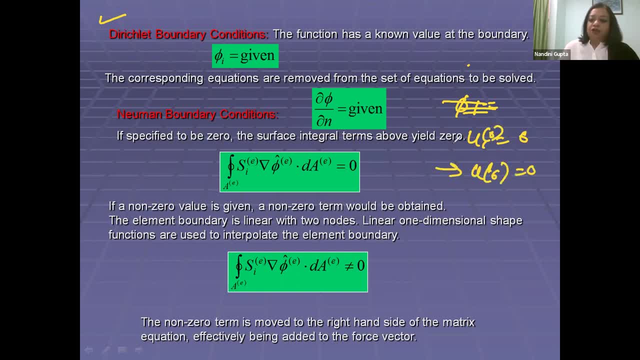 u one zero is equal to zero and then u six is equal to zero. So the solution variable was specified. that is a Dirichlet boundary condition. That is one option. In the other case, the rate of change of the solution variable across the surface or across. 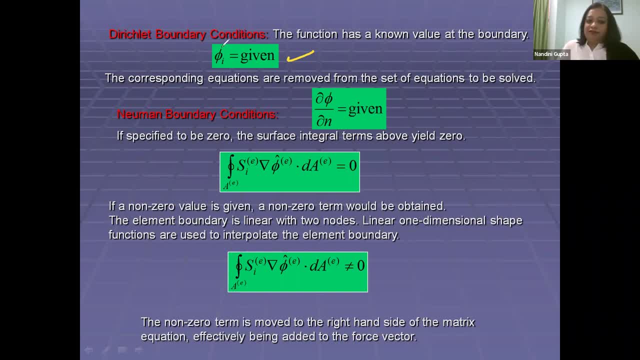 along the normal is given, which means it's: either phi is given- and I say phi i because any edge if you have, okay, if you have something like this, we are not really considering the entire line. we are considering this to be a conglomeration. 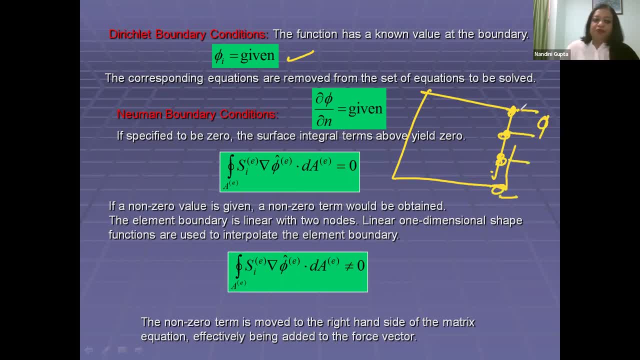 of points. So at every node along this boundary phi is given, So phi i is given. that is one option, which is the Dirichlet boundary condition. The other is that the rate of change of phi is given along the boundary, along the normal, in the normal direction to the boundary. this is given. 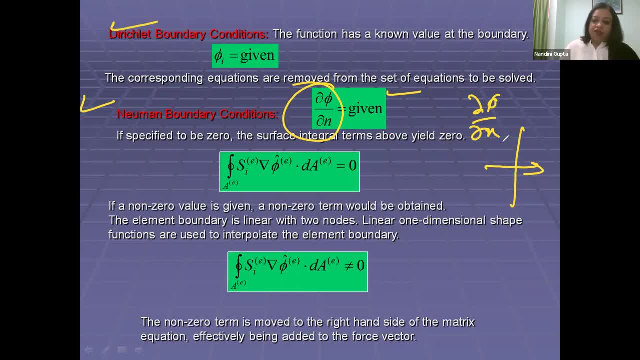 So these are the two possible boundary conditions: either Dirichlet or Neumann. Now, if you have Dirichlet boundary condition, you do not really need to evaluate the equation corresponding to the Dirichlet boundary conditions, which means, let us say that you have Dirichlet boundary conditions. 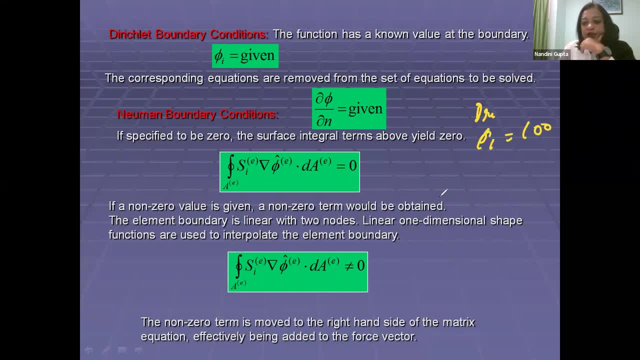 specified at node equal to 1.. So it's given, which means that no matter what your stiffness matrix is, I'll Ultimately you're going to impose a boundary condition, so you will do K1, 0, 0, etc. 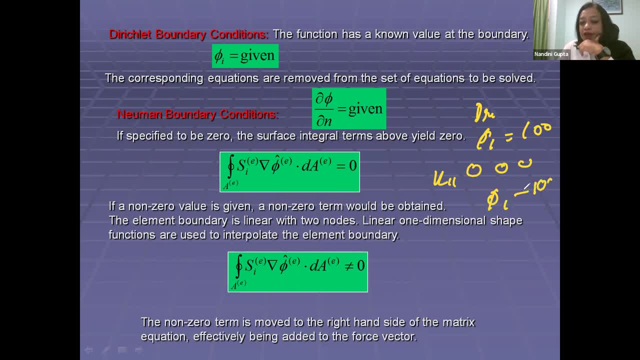 And you will force the value of phi 1 to go to the given value. So therefore you do not need to evaluate any term which has S1.. So in your equation if you consider that the first term has gone to 0, in your equation corresponding to S1,. 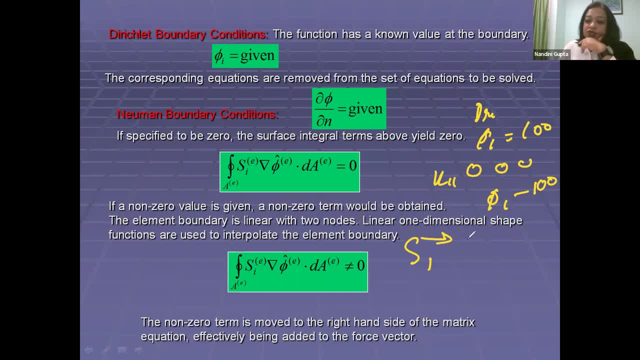 even if you, correctly or incorrectly, assume that the first term, remember what I said. I said that before obtaining the stiffness matrix, we assume that the first term is equal to 0. Now suppose the first term is not really 0. It does not matter, because you are not going to use that first term to evaluate anything. 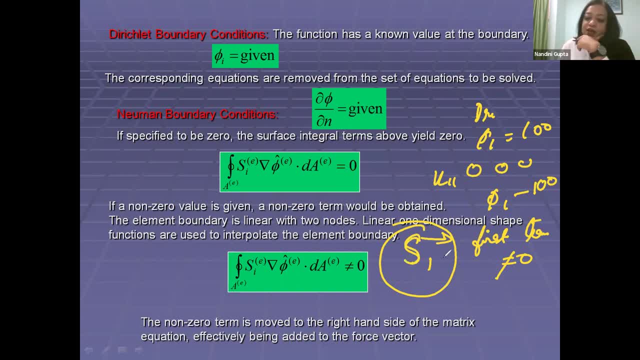 You are actually essentially going to remove that S1 equation from your. S1 will give you the value of phi 1.. You are actually going to remove that equation From your calculations, So even if it is incorrectly obtained, it does not matter. 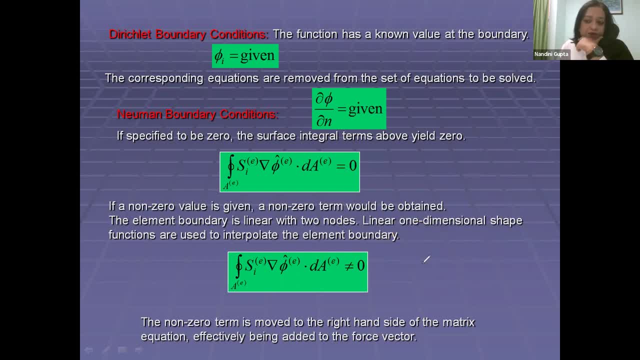 So essentially, those equations are not there if your Dirichlet boundary condition is given, because whatever Dirichlet boundary is given, you have the actual equations And those are the actual equations which will have to be satisfied Any stiffness matrix equation that you calculate, you are not going to use it. 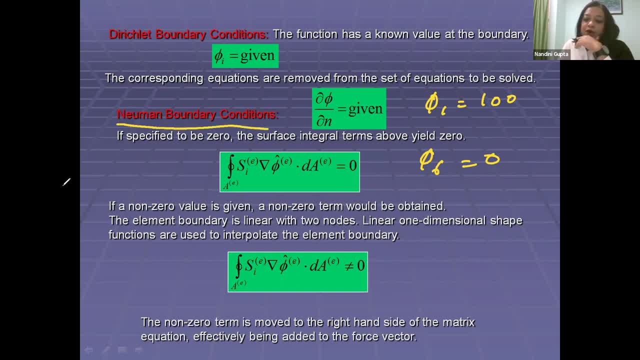 You're going to throw it away. And if you have Neumann boundary condition and if it is not specified, then the default condition, default hypothesis, is that del phi del n is equal to 0.. Let me give you an example. Let us take the parallel plate capacitor problem. 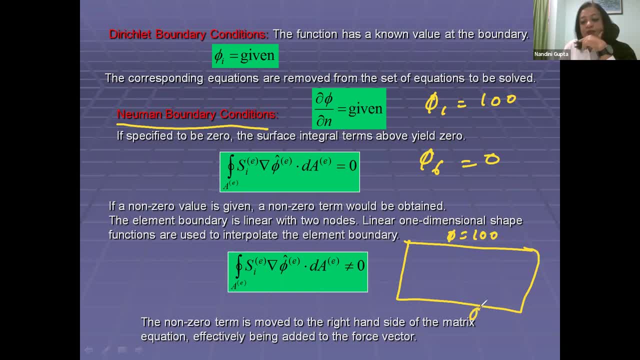 Now in the parallel plate capacitor you will have some Dirichlet boundary condition on the top plate and the low plate. Remember, Laplace's is a parabolic equation, sorry, elliptic equation. Elliptic equation means equation. the boundary condition has to be specified. 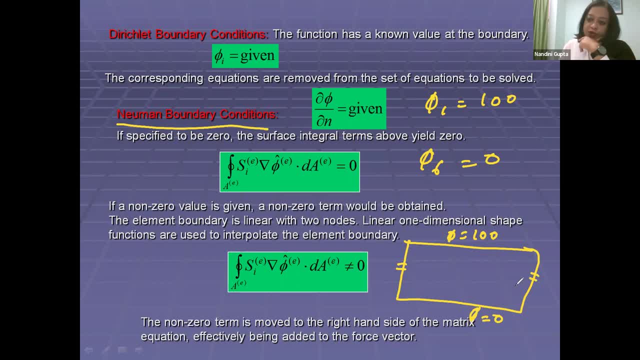 Around a closed boundary, so you need boundary conditions on these two boundaries. also, If this were a parallel plate capacitor, what would be the boundary conditions of the sides in terms of phi? potentially, What is the physical assumption? Remember, your mathematical representation of a problem has to come from a physical representation of the actual scenario. 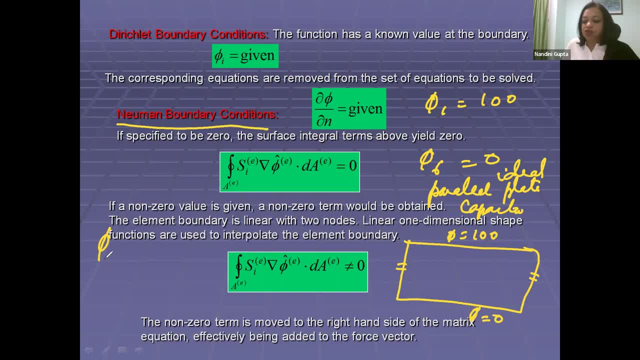 So what do you know about the boundary? What do you know about the potential at the boundary sites? The potential at the boundary sites is equal to zero. It will be zero. It will be Zero. What will be zero? The potential will be. 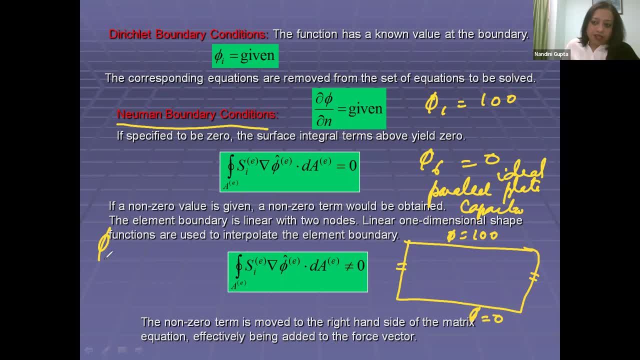 Potential will be zero. That is equivalent to ground condition, which we have on the lower plates. Why should we have ground condition on the side plates? That is not correct. What will be zero? Something will actually be zero. Ramanuj, you have done 634.. 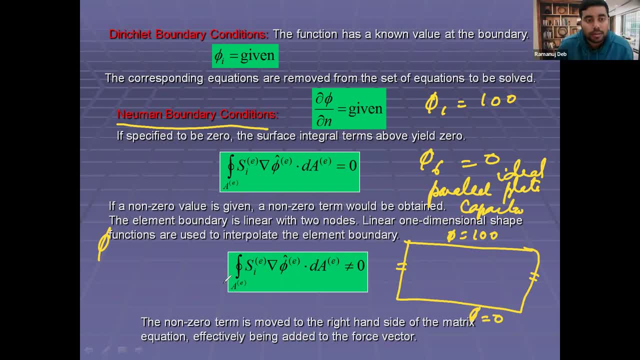 It will be fringing at the end. Come again, There will be fringing at the end. I said ideal. I said ideal. So if there is a, If there is a, If there is no fringing, what do you know about the potential? or maybe electric field at the edges? 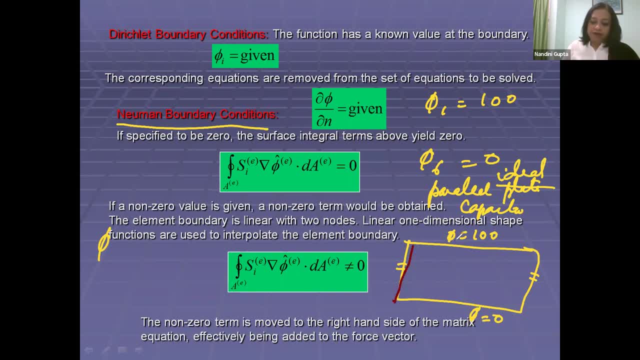 What do the electric fields look like? Lines will look like that. Let me draw it a little nicely: None gradient of Yes, Yes, hte. Ok, I'll do this. So any nodes here will have phi equal to zero. Any nodes here will have phi equal to 100.. 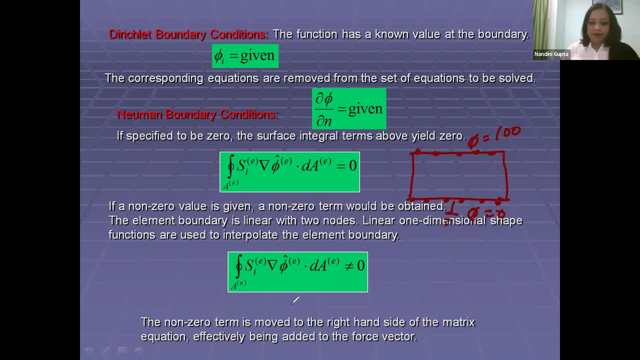 The sides. What does the field look like? I say no fringing. Yes, So the electric field will be parallel to the boundaries, right, Which means what will happen to the electric field in this direction, perpendicular to the sides. This is the side. 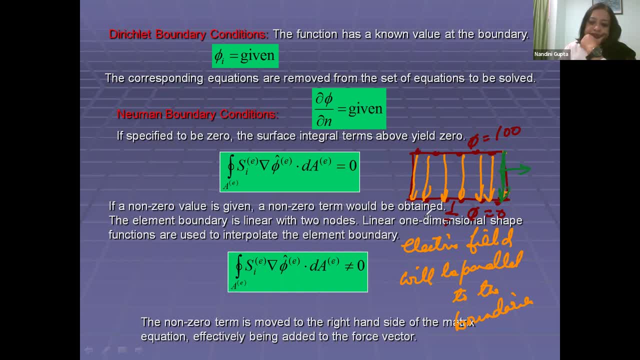 You have an electric field which is tangential to the side. The electric field is tangential to the edge, to the boundary. So what can you say about the electric field in a direction parallel to the tangent Zero, Zero? So E n is equal to zero. 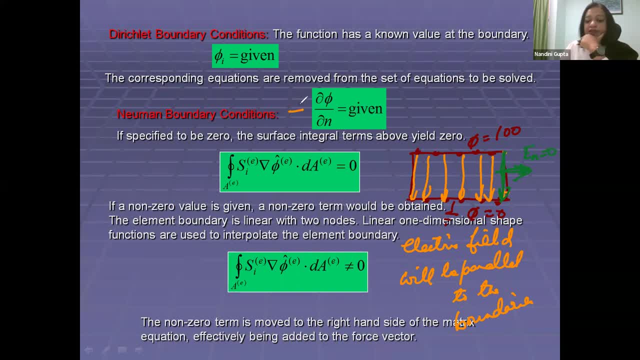 If E n is equal to zero, what is E? n Minus del phi del n? So del phi del n is equal to zero, right? So you might have. this is one example of a boundary where the Neumann boundary condition goes to zero. 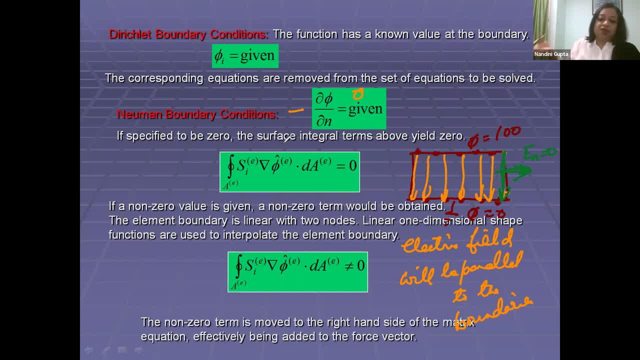 It is not necessary that it will always go to zero, but I'm just considering the case when it does. It does go to zero and I'm giving you an example where it does go to zero. Now, if it goes to zero, then the surface integral terms above should give you zero. 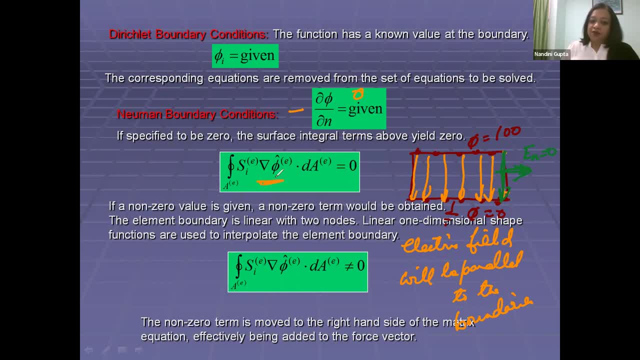 If del phi del n goes to zero, it means that this must go to zero, So this will go to zero, Isn't that? so This is being this is grad phi, Right? So if grad phi is zero, if del phi del n is zero, the grad phi into the normal dot product. 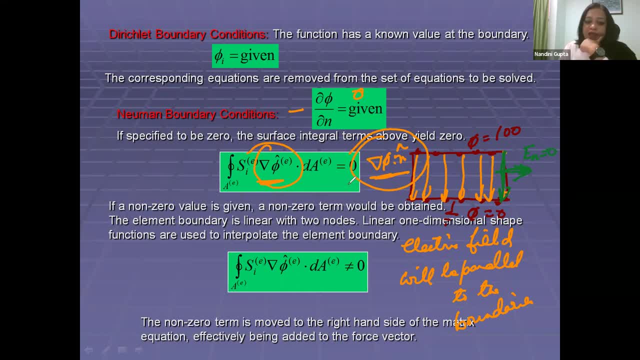 of the grad phi with the normal component will go to zero And therefore if you're integrating zero, you will get zero. So it means that if you have a Neumann boundary condition equal to zero at a boundary- we are talking about the outer boundaries here- 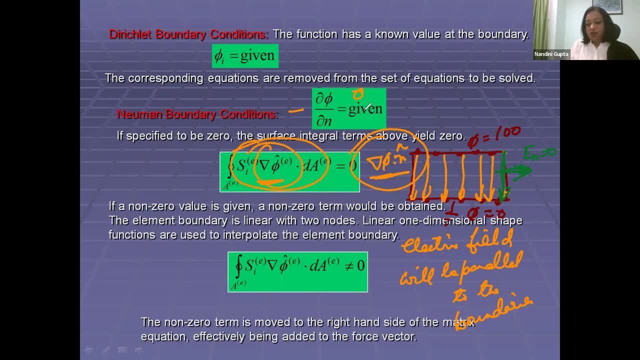 Inner boundaries. I don't care, because inner boundaries they will anyway cancel each other out. But if you have the outer boundaries, if the Neumann boundary condition is given to be zero, then it is true that the first term will go to zero, which is what we had as you. 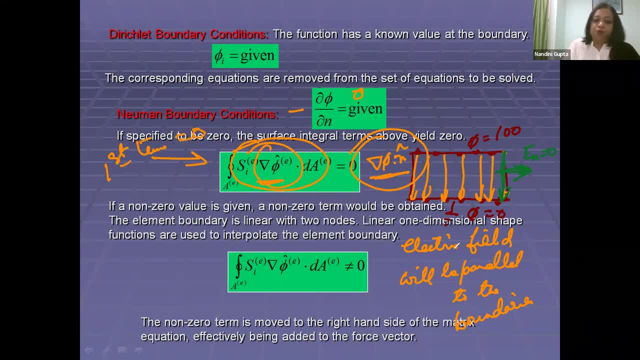 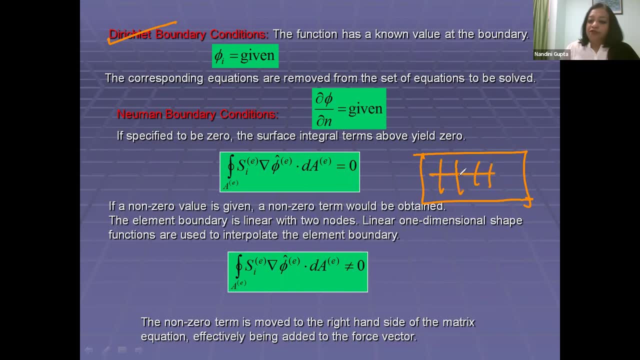 First term does go to zero. So what have we been able to prove? We have proved that, if so, if you have a domain, you do not need to evaluate the first term. in your equation of a residual equation, you do not need to evaluate the first term on. 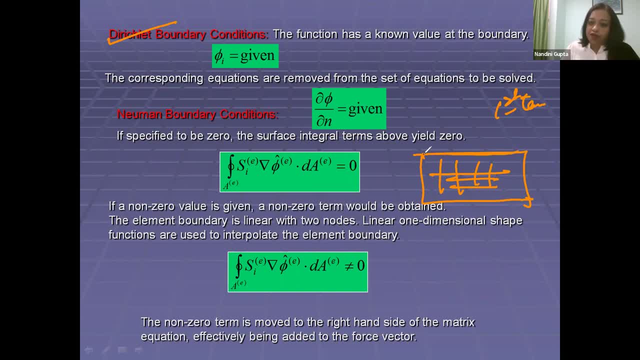 any of this. You only need to evaluate them at the external boundaries. Now, if in the external boundaries you have Dirichlet boundary condition, nothing matters, You can consider this to be zero, because you are anyway going to remove the equation from. 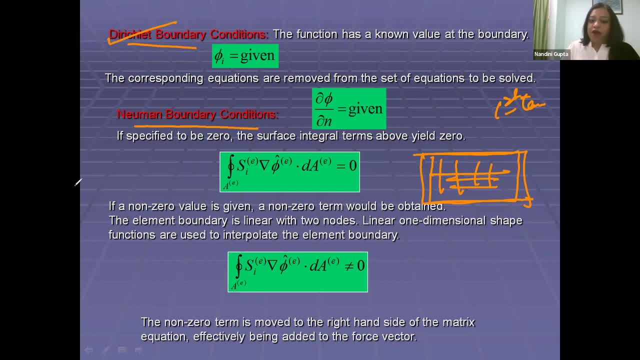 the reckoning. But if instead you have Neumann boundary condition and the Neumann boundary condition is given to be zero or can be assumed to be zero, then the first term actually does go to zero. So so far we are justified In taking the first term to be equal to zero, which is the question that Sandeep asked. 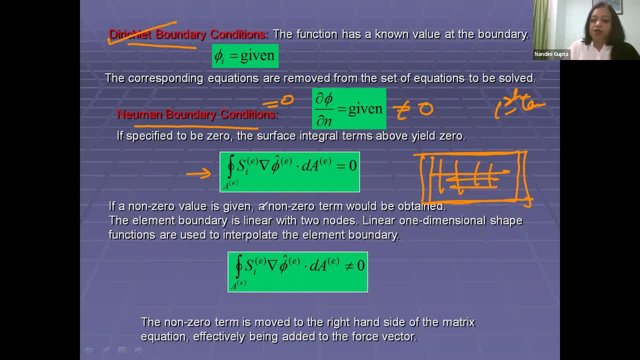 However, if Delphi, del n is not equal to zero and has a given value, then this integral has to be, cannot be zero and it has to be evaluated. But you can evaluate it because you can evaluate this will be known At that point of time, this quantity will be known and therefore you can, by integrating 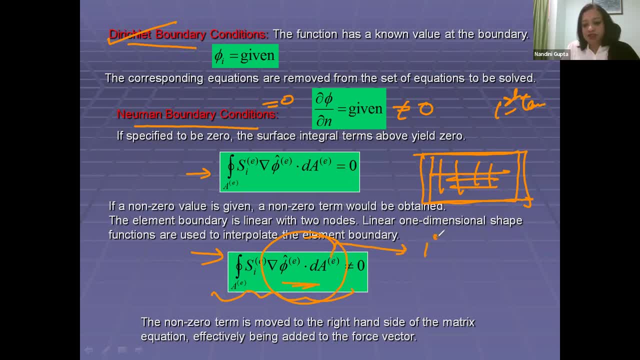 this quantity, you can find the term due to this first term Right And that first term. let us see what happens. then You'll have to wait till the circle keeps going round. So what will happen is you will have a situation. 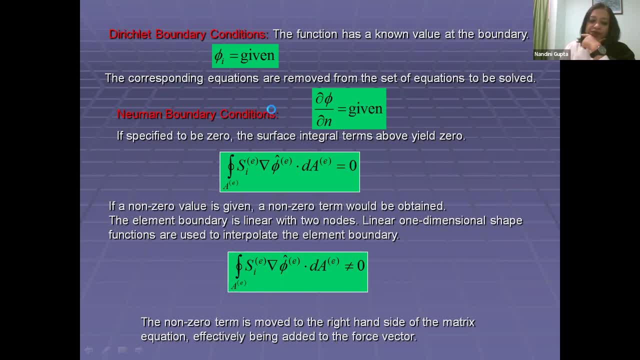 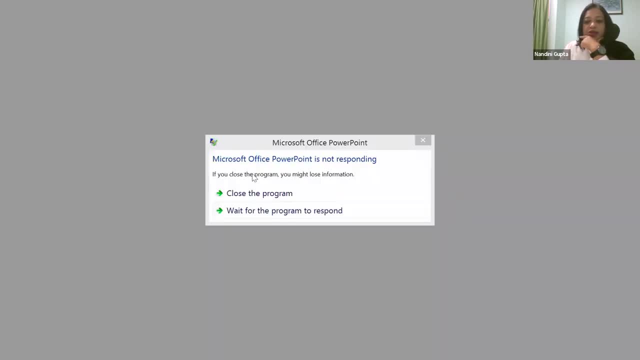 Where you have K. So what will happen is, if you remember, this is an equation which we are integrating over elements to get us the K phi equal to F term. Now, the first term was considered to be zero. If it is not zero, it will be a given. your grad phi dot n is a constant and it will be. 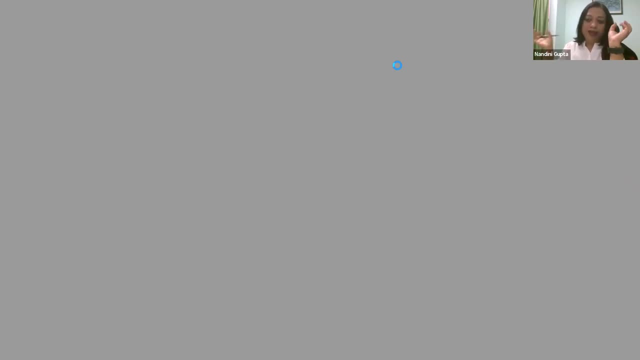 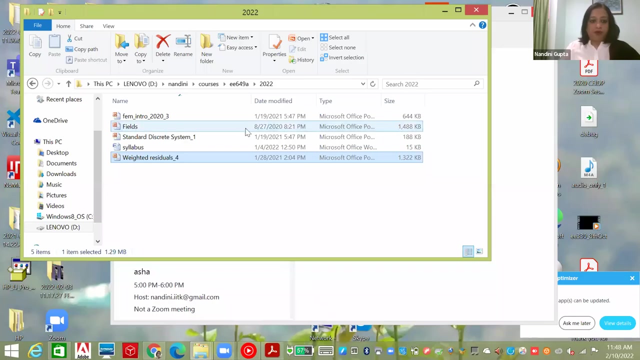 my, my, multiplied by the shape function, So you will get a term which does not have the nodal variables, And so you will get a term which is non-zero. Let me take it out: You will get a term which is non-zero. 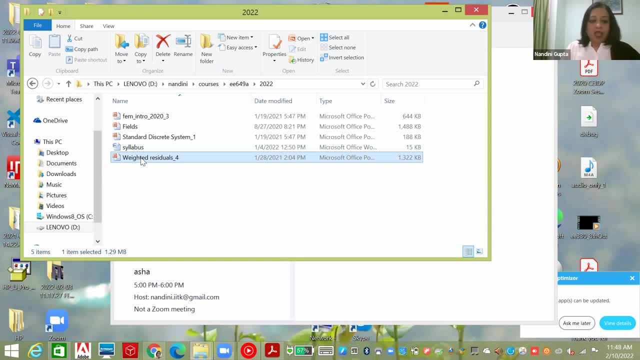 So you will get a term which does not have the nodal variables, And so you will get a term which is non-zero. Let me take it out. You will get a term which is non-zero. Let me take it out. You will get a term which is non-zero. 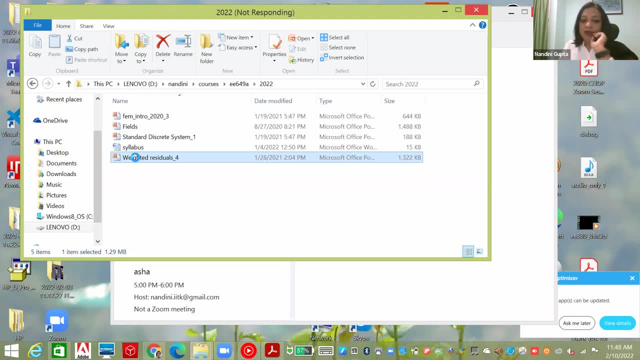 Let me take it out. You will get a term which is non-zero, And that term depends upon the given conditions. What kind of condition? If your flux is given, if del phi del n? OK, while we wait for this to open, which is taking. 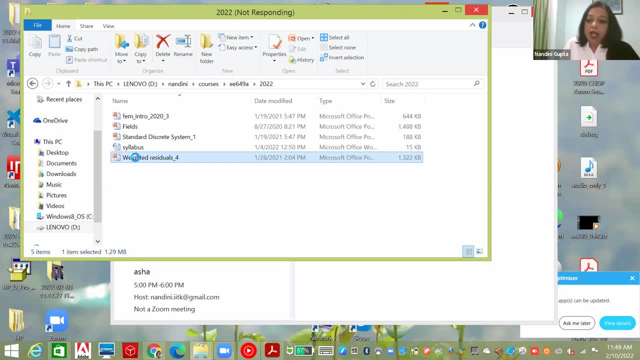 an infinite amount of time. I think my computer is playing up. What does it physically mean to say that del phi del n across a boundary is non-zero? What is the physical significance of that? What does it physically mean to say that del phi del n across a boundary is non-zero? 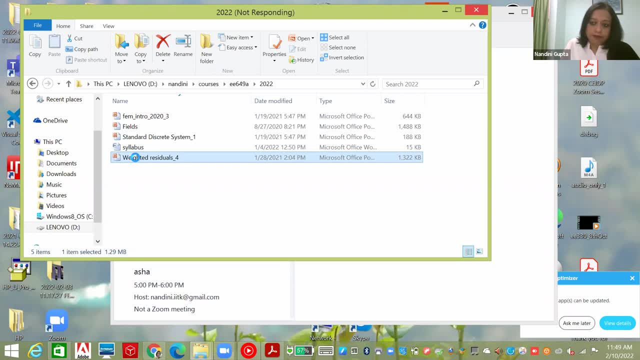 I guess my computer is playing up. There are fluxes there, Some flux is there passing through, Some flux is cutting through the surface, Exactly so, And you essentially need to know that flux quantity Before you can evaluate it. you need to know the flux quantity. 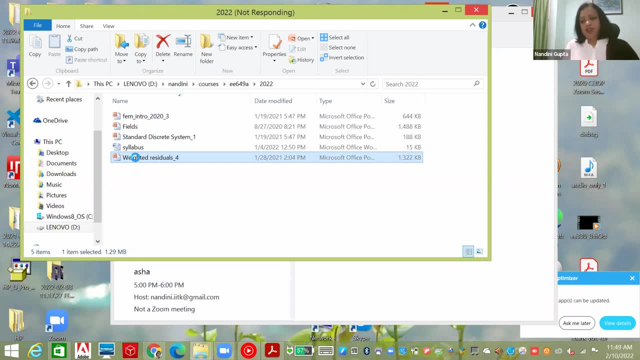 So that is specified. Can you think of a situation where you have an eigenvalue and you think of it today, Right, Where is that? Let me think of this parallel plate capacitor and there is a flux going through the surface. Maybe you have placed the capacitor in an external field. 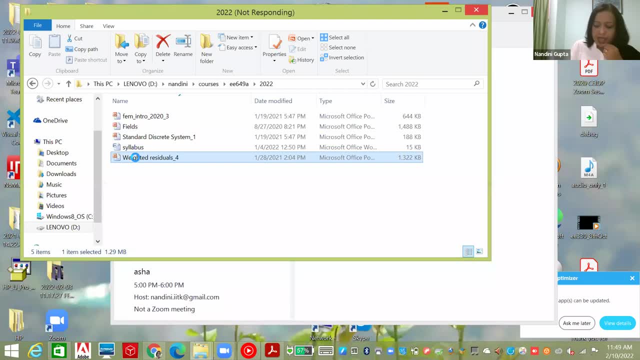 where there are flux lines already cutting through the surface. So that kind of situation where it is like a forcing function, it is like an additional source of electric field. If you only have the Dirichlet boundary conditions, you only have the Dirichlet boundary conditions, you have the Laplacian field. 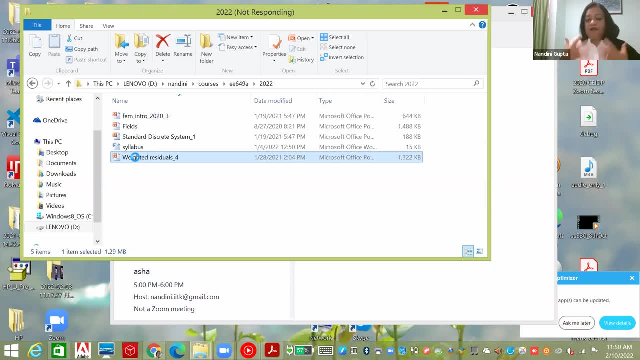 If you have rho, you have the Poisson field. If you are specifying that there is a flux cutting through the surface, it is probably coming from some other source, It is a possibility. So it is like there being a second source, so a second forcing function. 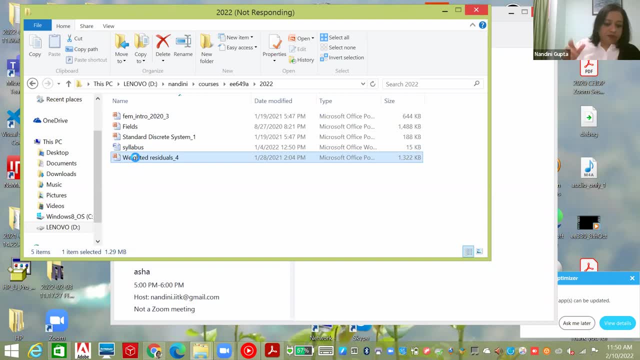 So when you evaluate this, I think I'll have to close down the meeting and reboot my computer before we can move forward. When you evaluate this, what you will see is you will have a term which does not have the nodal variables and therefore can you move to. 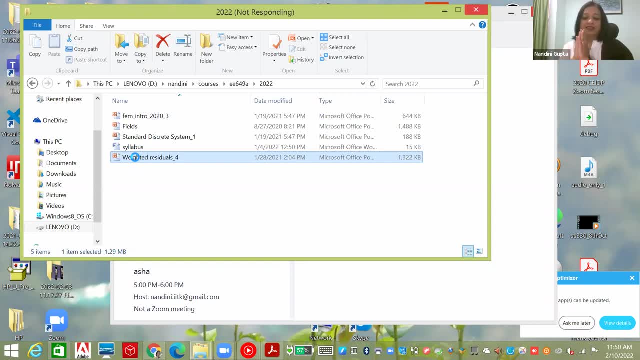 the right-hand side of the equation And in the right-hand side, therefore, it will contribute to the force vector. So it is like an extra force forcing function in your problem. It is an extra source And therefore this term will then contribute to the forcing function. It will not contribute to. 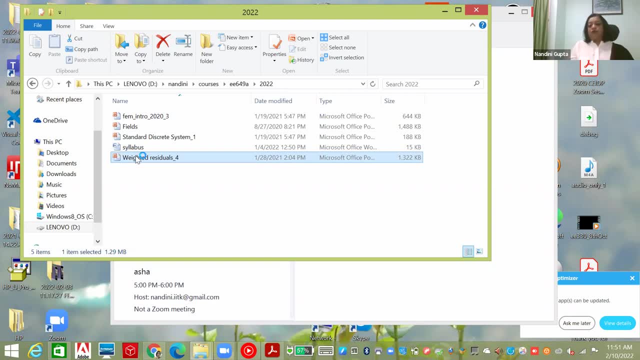 the stiffness matrix. So what have we discussed so far? I have evaluated for you that I had already done: how to evaluate the shape functions and set up the equation so that you have the local stiffness matrix and you assemble it into a global stiffness matrix. Now, in doing this, the terms that 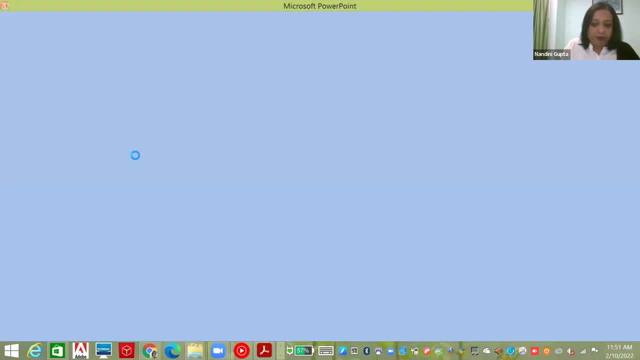 we use are the second and third terms after algebraic manipulation. So the first term is the интерес of algebraic manipulation. The fourth term is taken to be Z. First term will always be taken to be zero, unless you have a Neumann boundary. 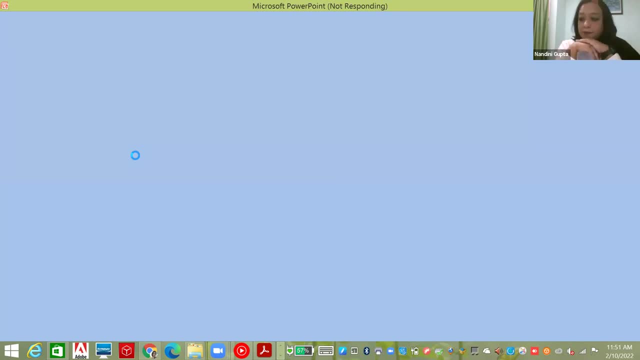 condition specified at a boundary. The reasoning behind this is this: that at every internal boundary, this, this is conver. The first term is a conteúdo integral, So therefore it has to be taken along the boundaries of the elements and along any internal boundary This will be. 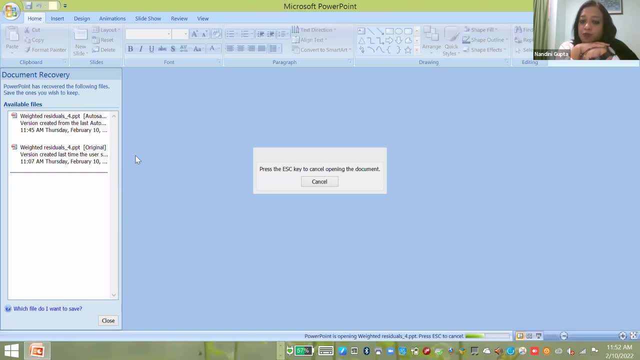 adjacent to more than one element and therefore the contributions from the adjacent elements will cancel out and will not contribute anything. so therefore, we do not need to evaluate this first term over any of the internal boundaries. they, however, have to be evaluated over the outer boundaries. when you consider- i don't know what's happening when you consider the outer boundaries. 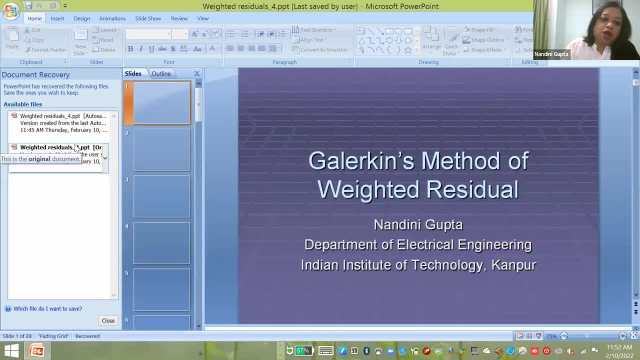 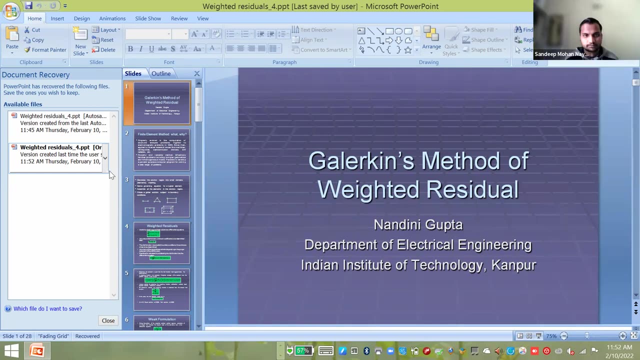 the possibilities are two. you may have a Dirichlet boundary condition or you may have a. you may have a Dirichlet boundary condition or a Neumann boundary condition. if it's a Dirichlet boundary condition, if you make the term go to zero, it does not matter. 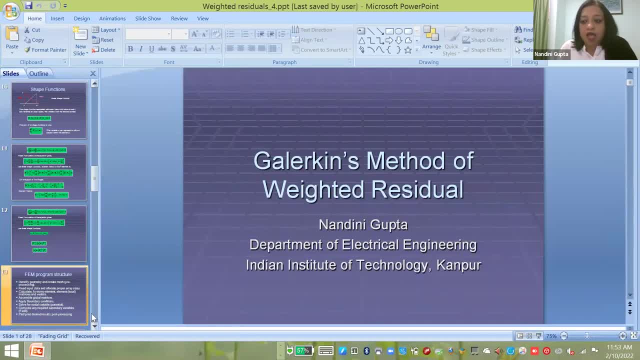 because any equation at the dirich at that boundary will be replaced by the given value of phi. so, ultimately, the equation that you're going to use is always already known: phi1 equal to 100 is what you're going to use, no matter what contributions you. 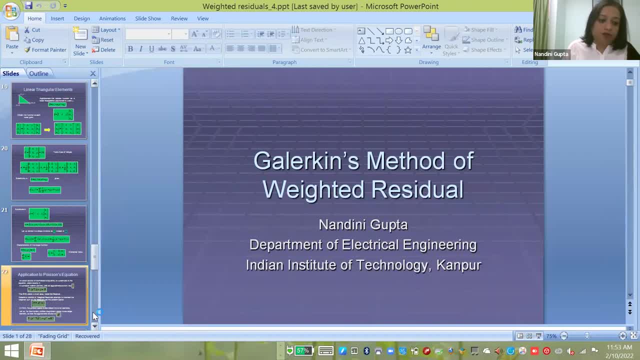 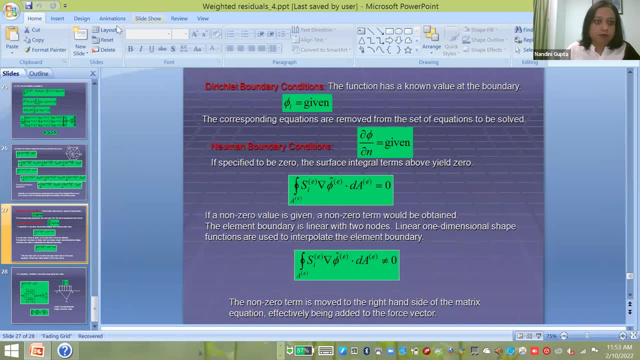 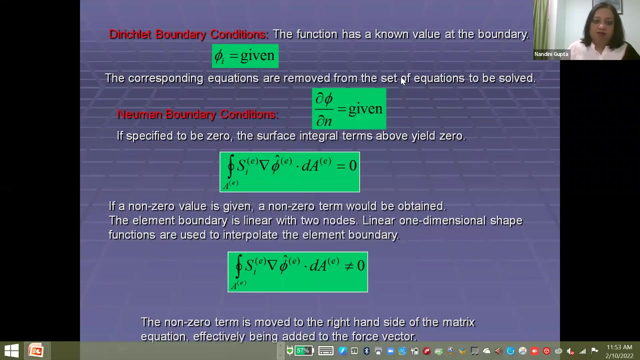 get from the stiffness matrix or otherwise, so you don't really need to bother. but if instead you have, if instead you have Neumann boundary condition and Neumann boundary condition is equal to zero, in that case also the first term goes to zero. if you add public Feh i I2 to that value. 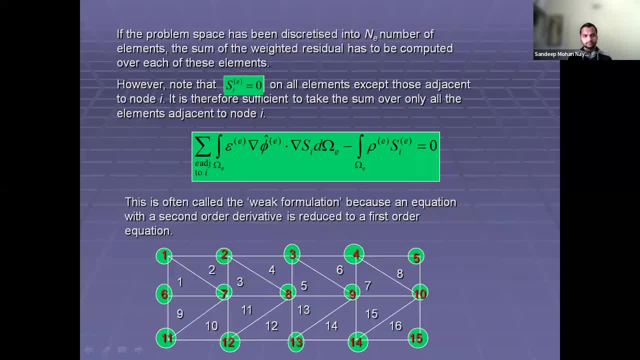 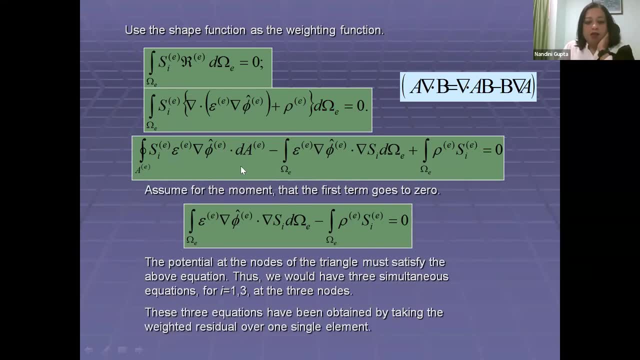 I2. Gregor, go ahead and put the over factor. this is the term that we were talking about, but I cannot. I noted, okay, I'll have to wait. so this is the term we are talking about, but we have to look at that here. all right, I'm going to start by writing a quote. 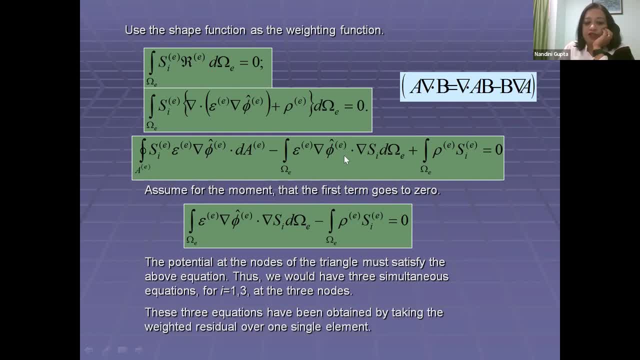 eventually. but I can do that because of invisible boundaries and so on. so I'm right again. this about this second and third term contributes to my stiffness matrix. now, if it is Dirichlet, I can make it go to zero without any error creeping in. if it is Dirichlet, Neumann boundary condition. 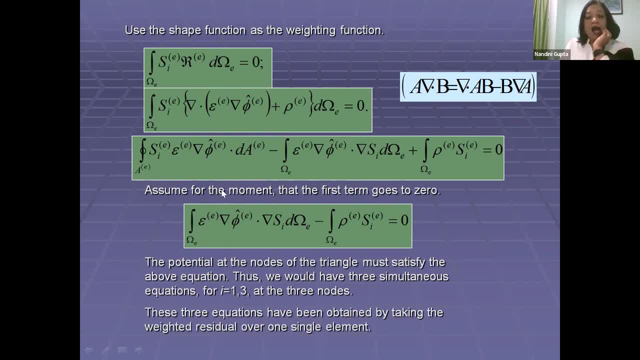 equal to zero, then, also, this actually does become equal to zero. however, it does not become equal to zero if I have a specified boundary conditions. if I have a specified boundary condition, then what I need to do is I need to evaluate this term and I will be able to evaluate this term. 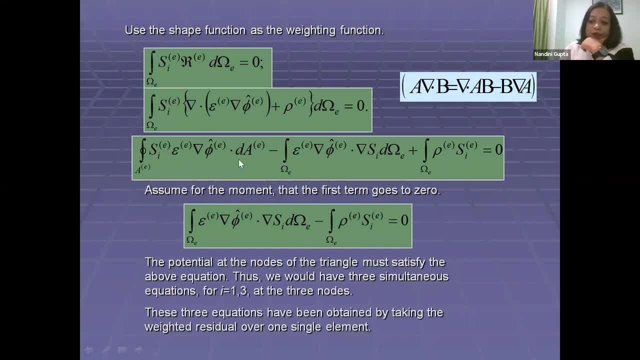 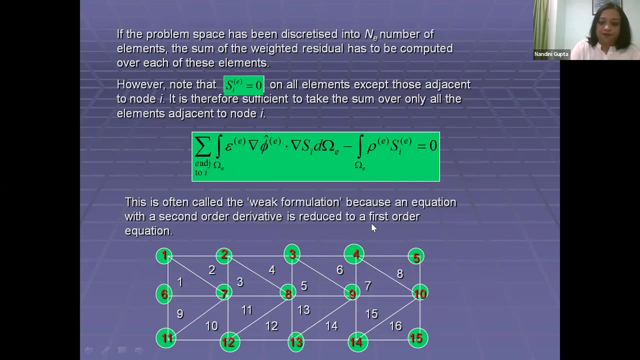 because del phi dot n over a boundary will be specified and this will contribute a term which will not have phi in this equation and therefore it can be removed to the right hand side and it will add to the force vector. so this is what will happen: you will have a term which is: 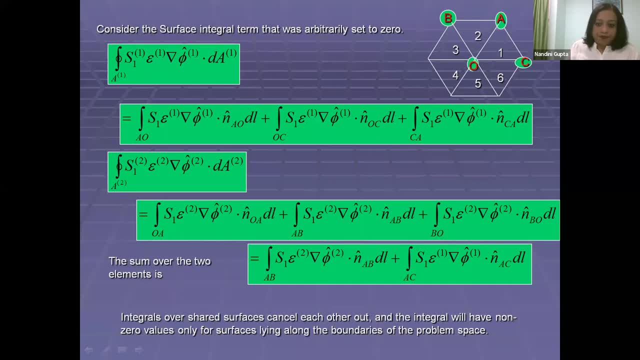 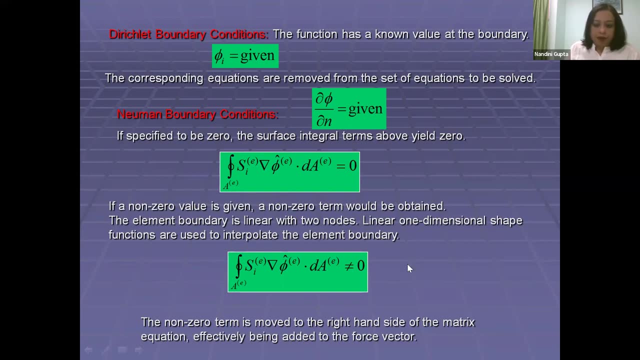 adding to the force vector. so Want you to see this. So the non zero term is moved to the right hand side of the matrix equation, effectively being added to the force vector. the same thing will happen if you have different values of permittivity. if you have different values of permittivity, it will result in a dn1 not being equal to dn2. 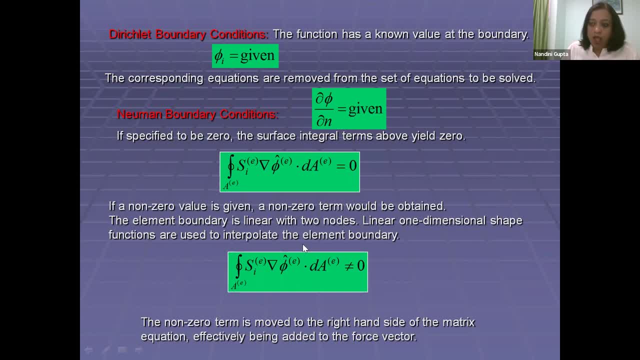 boundary will not be equal and you will have to know the inequality. if you know the inequality, you will be again you be able to evaluate the term. so, both in case where you have del phi not equal to zero, grad phi not equal to zero, or you have a situation where epsilons are not equal, 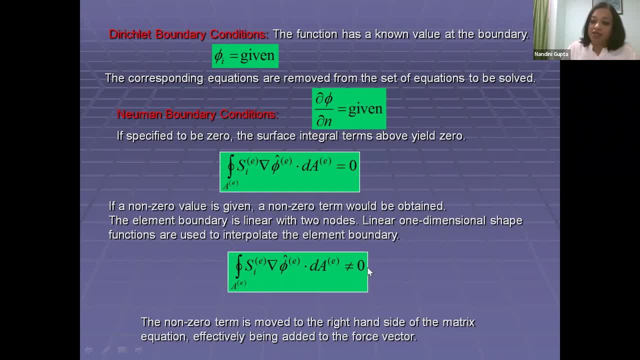 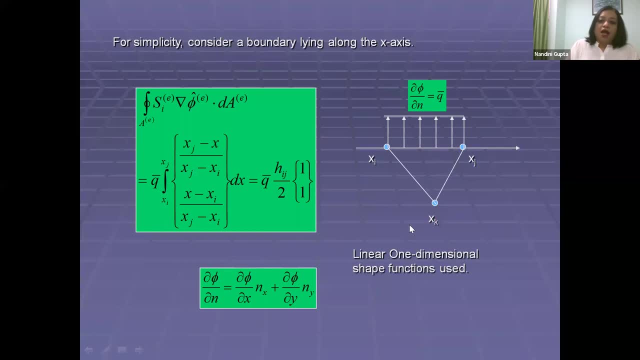 across the boundary, you will have some term which can be put into this integral and can be evaluated right. I'm giving you an example here how the term will be evaluated. let us consider a case. let us say this is a fictitious, this is a fictitious boundary. and let us say along this boundary you do not have Dirichlet. 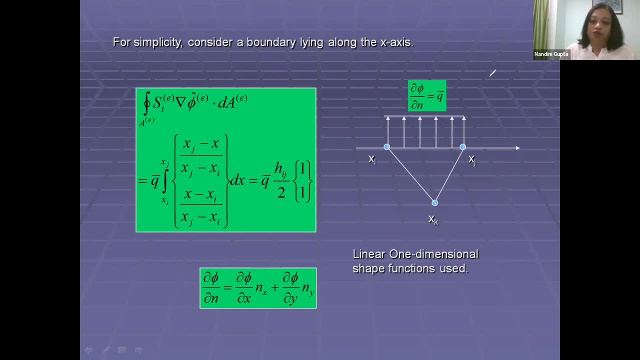 boundary condition. you do not have Neumann boundary condition equal to zero. you have Neumann boundary condition not equal to zero. you do not have Neumann boundary condition not equal to zero. case: to evaluate you must know the value. so this is your flux. let's say q bar is your flux. so if 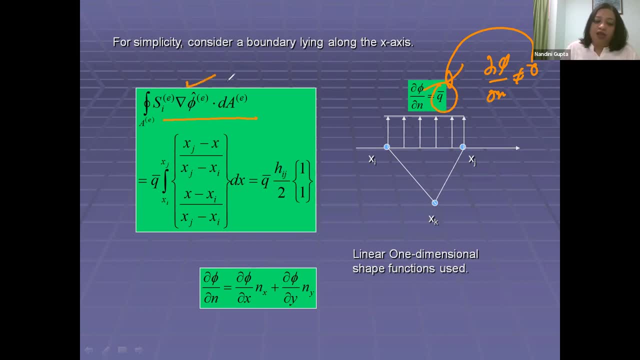 you are evaluating this and if you evaluate grad phi and d, this is x. so, uh dy, your normal is in the y direction, so that is why i have taken the edge along the x direction. you get this term and this, you can see, also contributes to a constant multiplied by the flux vector. so, as i said this, 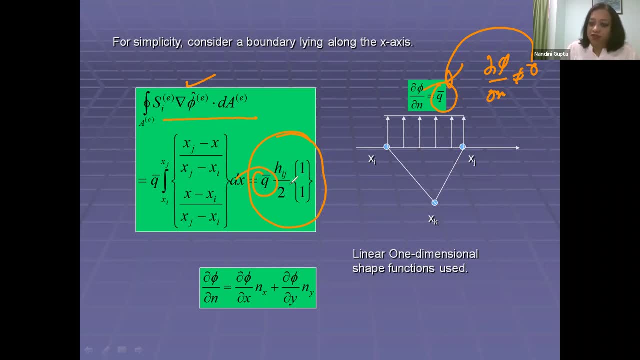 will give you a term which is in terms of constants and therefore it will add to the force vector. this is for a case where the boundary is along the x direction. if, instead, you have an arbitrary boundary which is neither in the x direction nor in the y direction, then you're in. 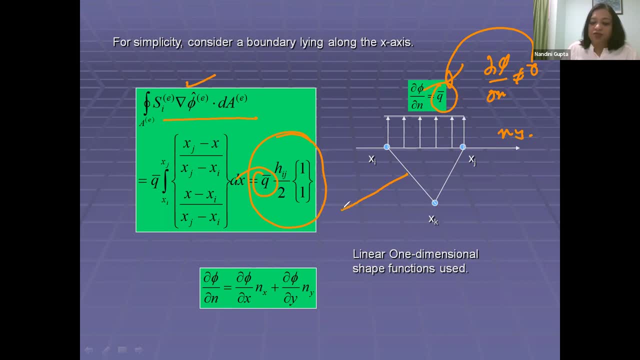 this case, your normal is in the y direction. in this case, for any arbitrary direction, you will have some component of this q in the x direction and some component of q in the y direction. you will have to know the component in the x direction. you will have to know the component. 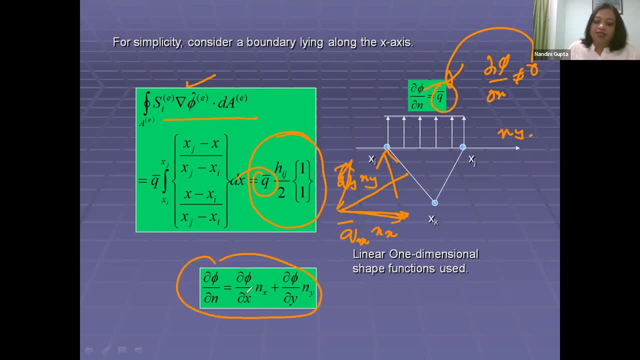 in the y direction, and then del phi del n will be del phi del x, nx, plus del phi del y, ny, and this will have to be put in the equation and evaluated. that's not a problem. so is it quite clear, because with this i think we stop our discussion on two-dimensional finite element formulation. that's. 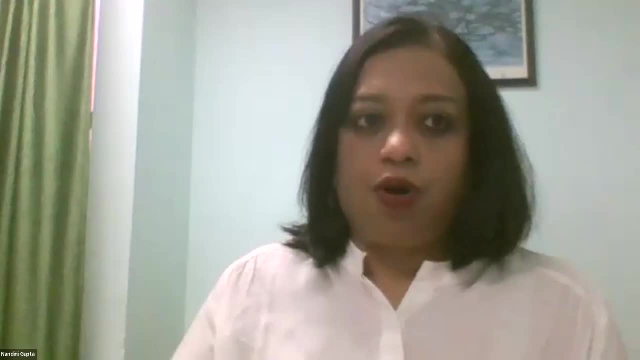 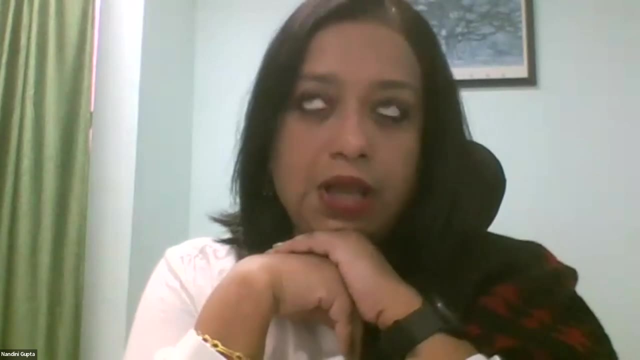 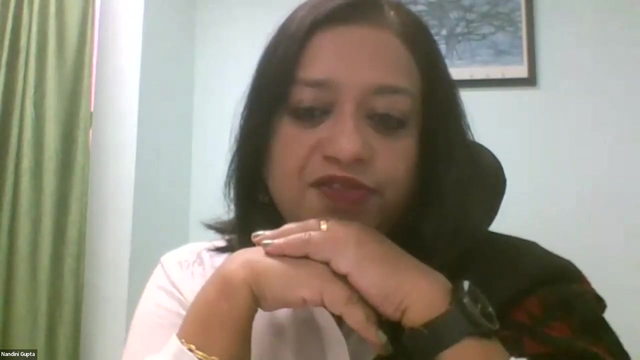 right? so, uh, let me tell you what we have done so far. we will start with something else in the next class. really, i think, yeah, we will start with isoparametric elements, but before that, let us conclude what we have done. what we have done so far is we have taken a one-dimensional problem. i have taught 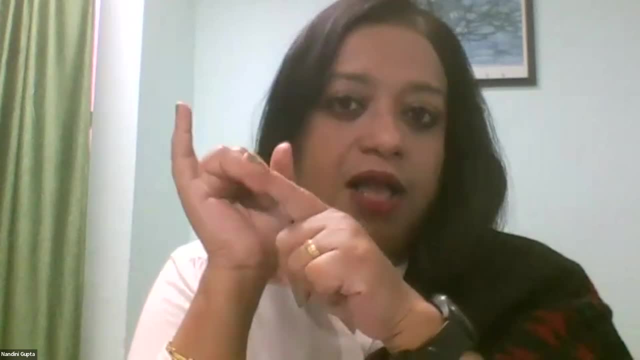 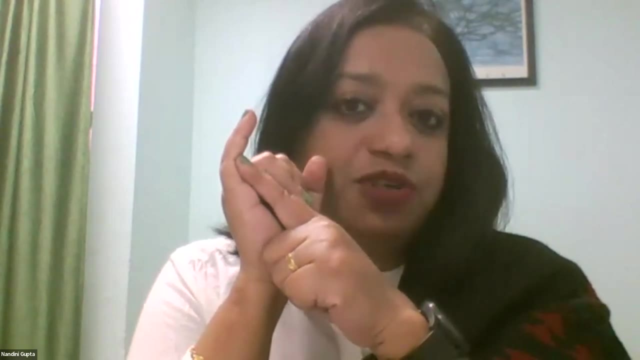 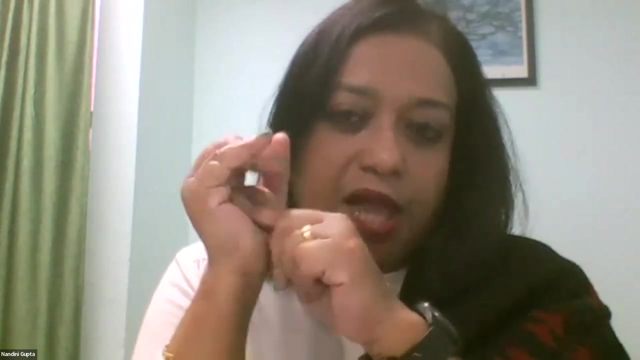 taught you the method of weak formulation. i have taught you the method of weighted residuals. you have learned to apply the method of weighted residuals when you consider a one-dimensional problem and the kind of element that you use is a linear, one-dimensional, linear, two-noded element. i have 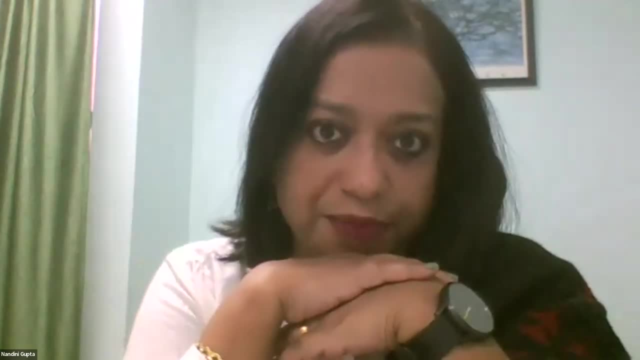 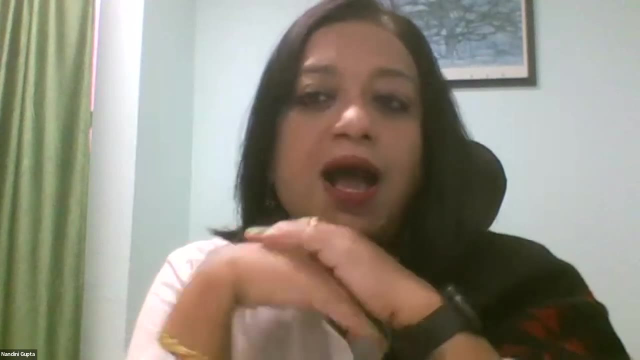 next extended our understanding of this to a two-dimensional problem. whatever i have taught you can be applied to any two-dimensional equation. i have taken the case of laplace's equation because we are the first kind of fields that we learn to solve in this course is the. 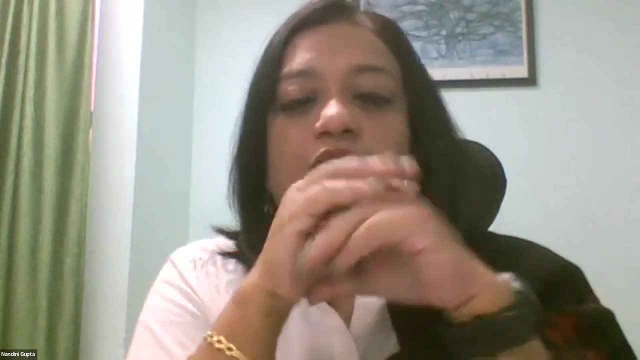 electrostatic field problem, which you have already revised. so i have taken the electrostatic field equation, which is your laplace's equation, and i have taken the electrostatic field equation, which is your laplace's equation, your laplace's equation or poisson's equation, and i have illustrated how grouped. 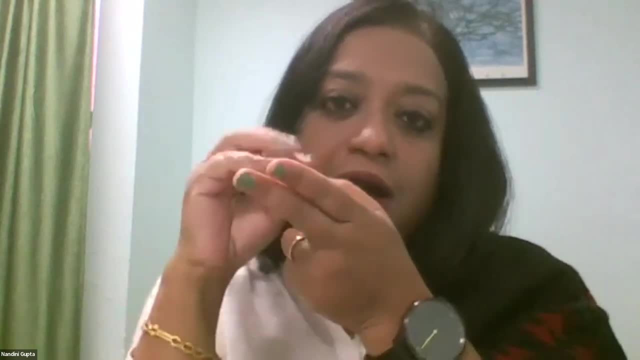 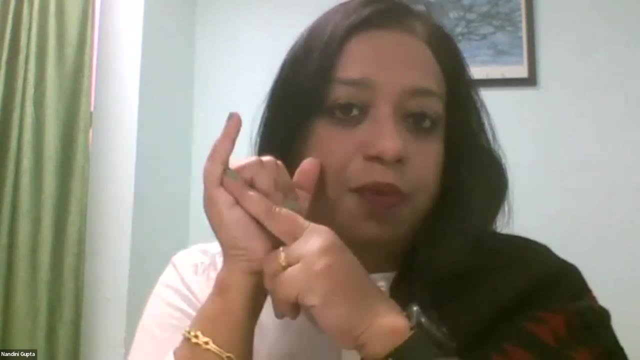 or poisoned. Angelina's equation- and i have done a little bit of analyse on that and you dough- formulates a two dimensional finite element problem. using this equation- but you are now in a position to do the same exercise- can actually produce the two-dimensional fit at 10 degrees. 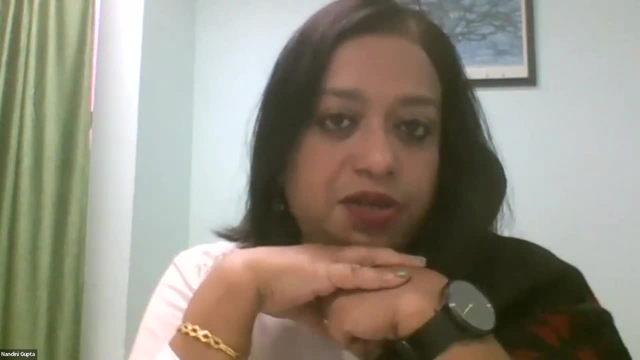 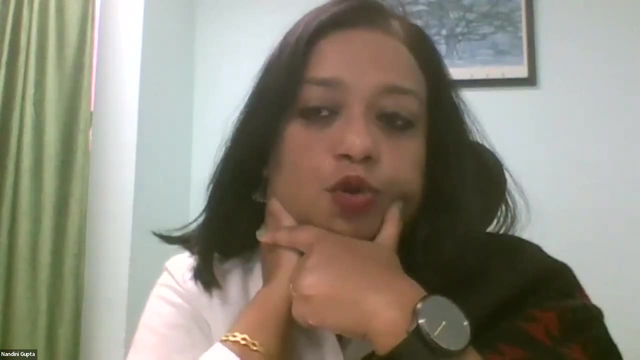 in the middle of the equation for any other equation also other than laplace's equation. in doing so, i have also illustrated to you a very simple two-dimensional elements, which is the linear triangular element, three-noded triangular elements we have so far: Orchestra of the Lady with ÖT's and some others. I have really taken a lot of interest by looking at it, and so I am very interested also in observing these three. 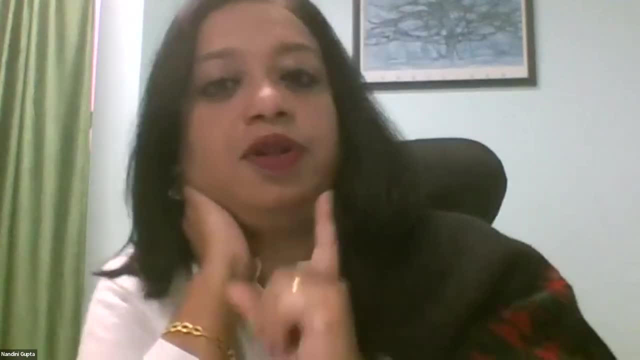 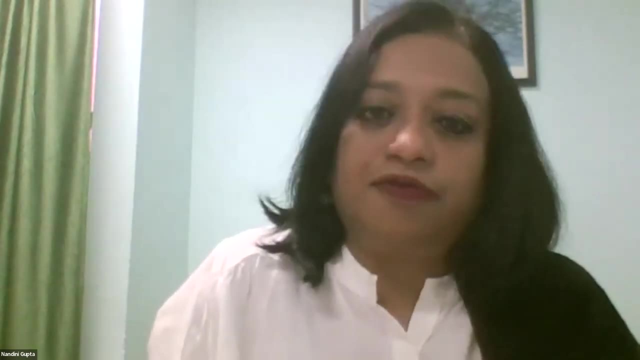 noted triangular elements, which is the linear triangular element, three-noded triangular element. we have only use the linear triangular elements. For the linear triangular elements, I have given you the weight functions. I have weighted you for the. I have found the weight obtained for you, the weight. 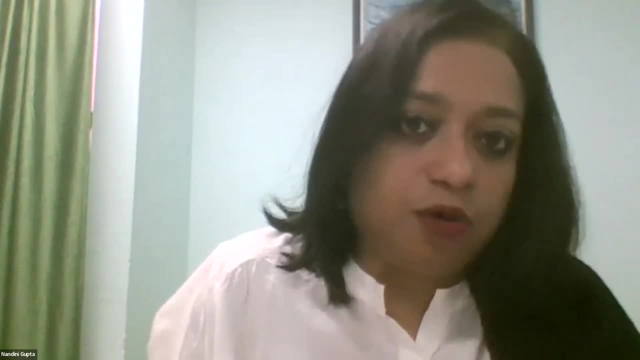 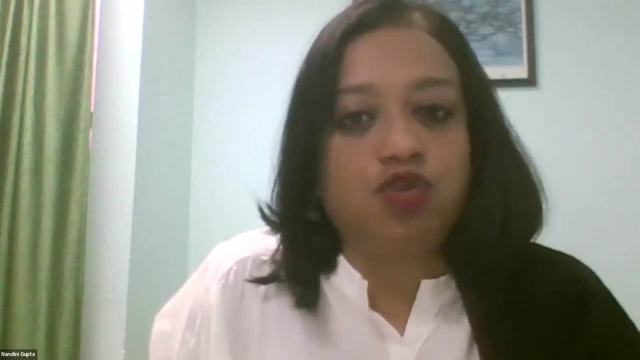 functions and you understand that the weight functions that we use in the one-dimensional problem as well as the two-dimensional problem ensures that the trial function that we choose for every element is a linear function In one dimension, linear in one, linear in x in two. 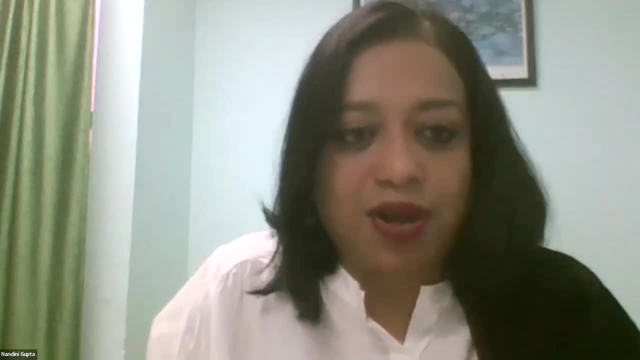 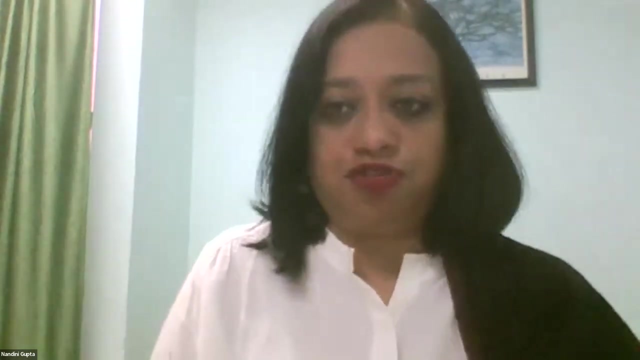 dimensions, a planar function that is linear in one x as well as y. I have also shown you how to handle the boundary conditions Right now. I'm not setting you this assignment at the moment because you're already doing one assignment Right now. at the moment, you are in a position. 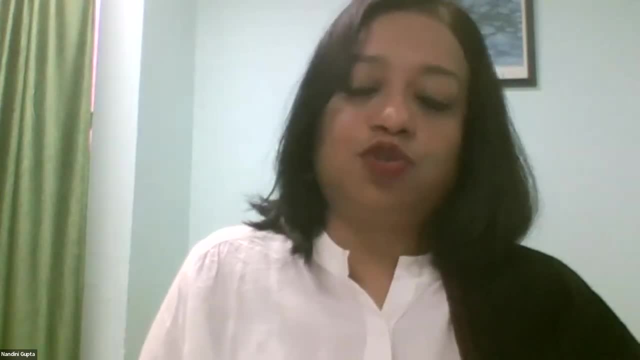 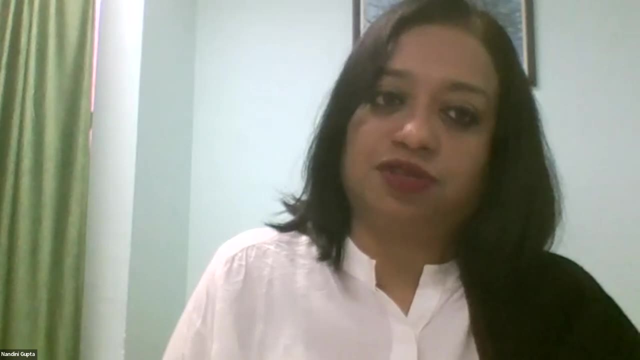 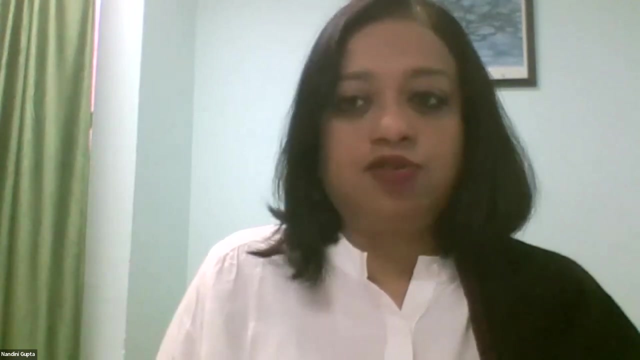 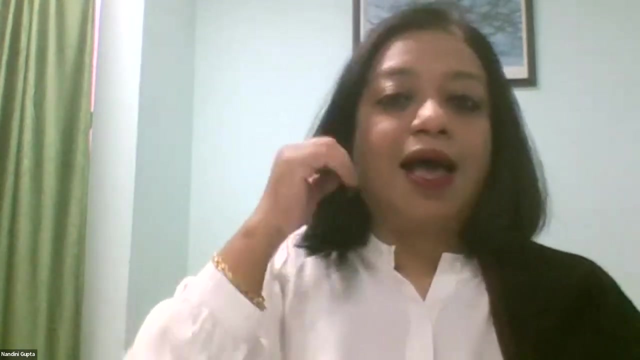 to write a MATLAB program to solve a simple partial differential equation or a simple electrostatic field problem in two dimensions. All of you agree with this. Now, so far, what I have done is I have only considered two simple kinds of elements and I have given you the weight functions I have not obtained. 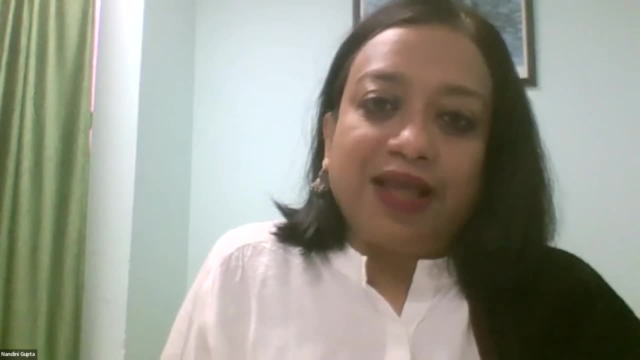 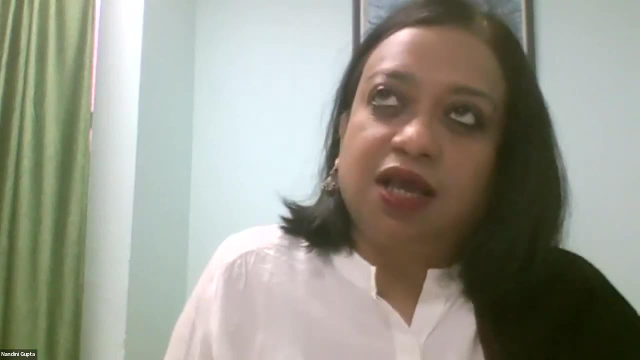 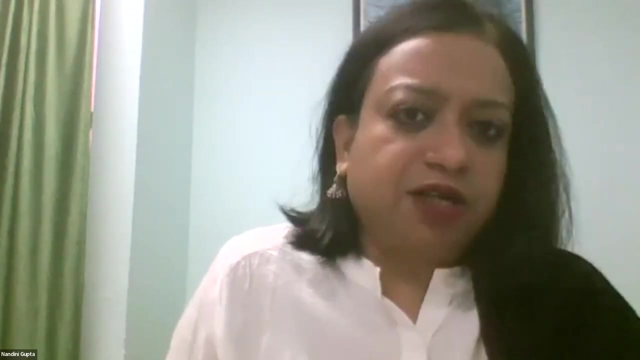 the weight functions for you Now in the next class. I want to go a little. okay, what we will do is in the next class. how many classes do I have before your midterm I have next week? Do I only have four classes? Okay, then I will not do magnetostatics. We will. 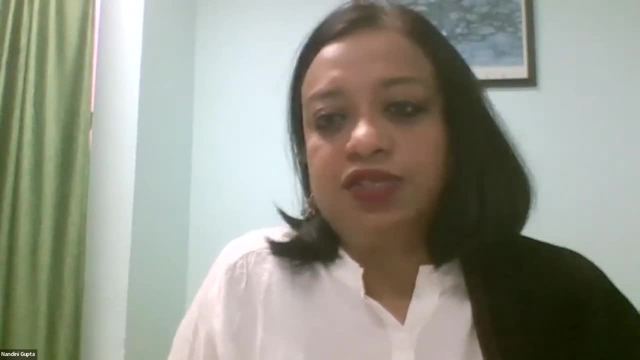 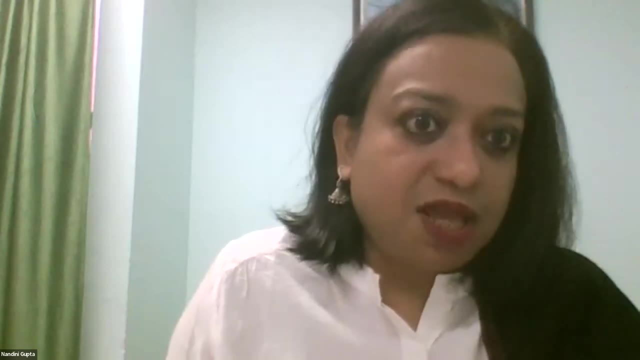 do magnetostatics after the exam. So what we will do is what I will do is I will give you a more formal understanding of how we choose the elements and once we choose the elements, can we obtain the weight functions without me telling you how to do them? 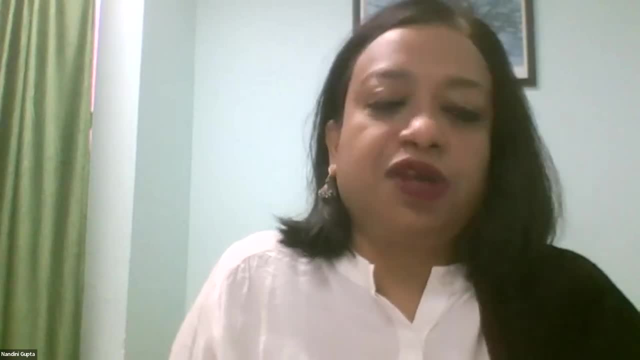 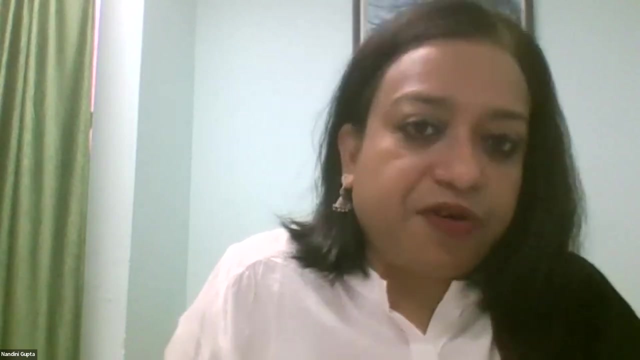 Before we go there, you really need to revise whatever has been taught so far. Much of it is repetitive. So if you can do the assignment I have set you, the rest is just an extrapolation of that. but I need you to be comfortable with whatever we have covered so far before I go ahead.